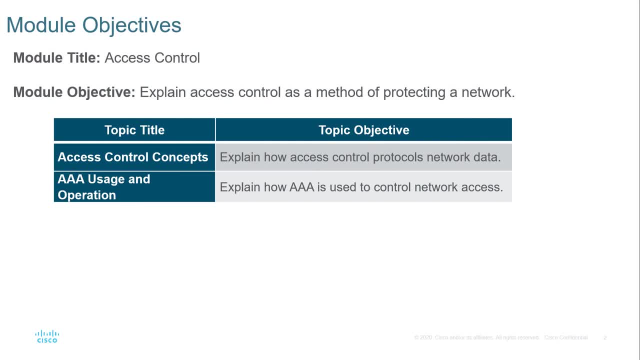 Basically explaining how access control works, How access control protocols actually function, And we are going to be looking at AAA- The usage and the operation. So let's go ahead and jump right on in Access Control Concepts. Normally you look at the CIA triad. 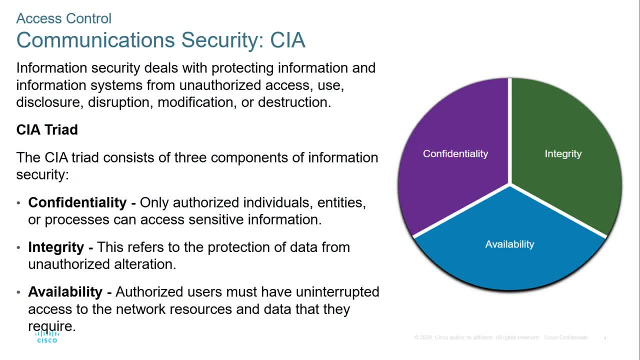 Confidentiality, Integrity, Availability. Confidentiality is keeping information confident and only allowing access to them to those that need access. Integrity refers to the protection of that data By allowing access to that data. Okay, Unauthorized alteration. Now the alteration can happen in motion, in transit, in storage, in use. 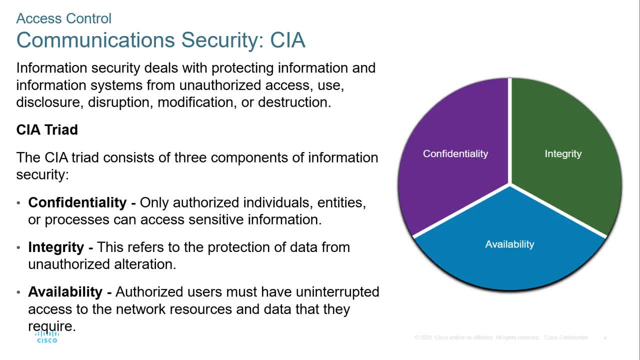 All of that should have a certain level of integrity, meaning that it's not modified at all Inappropriately. Again, those that are authorized to alter it is slightly different than those that are unauthorized to alter it. And lastly, is Availability, And that is essentially having 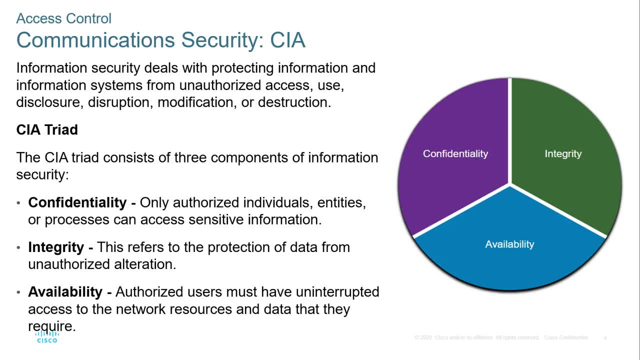 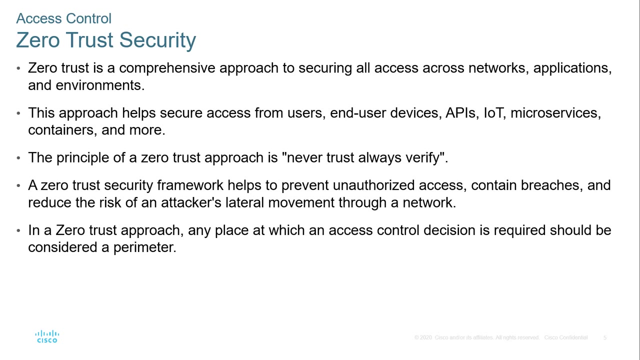 Access to a resource when you need, access based off of your authorization. If you are an authorized user and you should have access to it when you need it. This provides the backbone of basic information security. So we also have what's called a Zero Trust Model or Zero Trust Security. 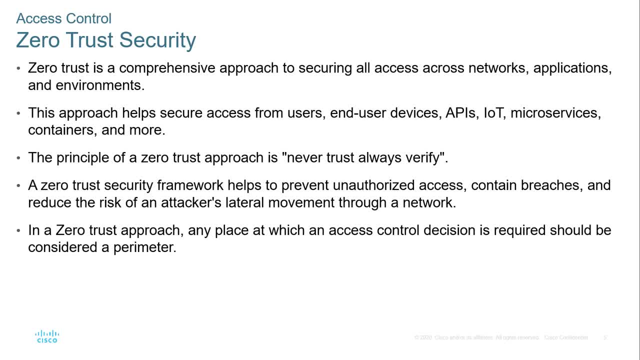 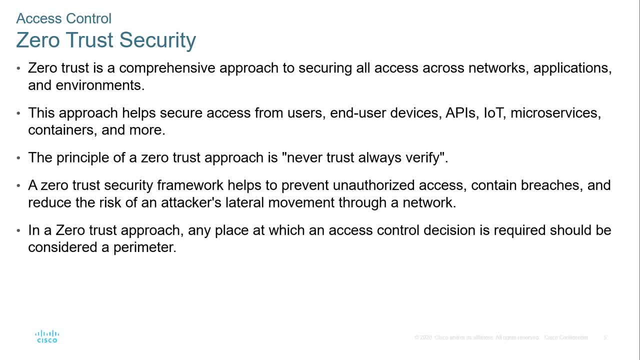 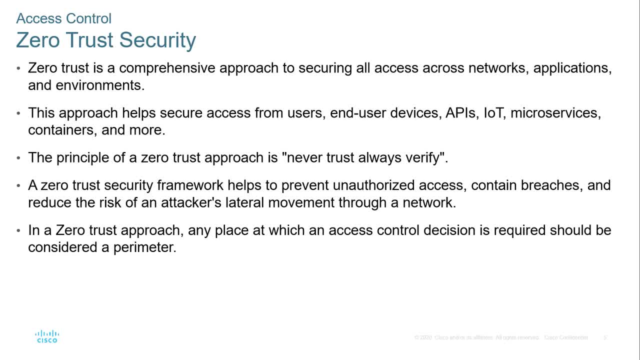 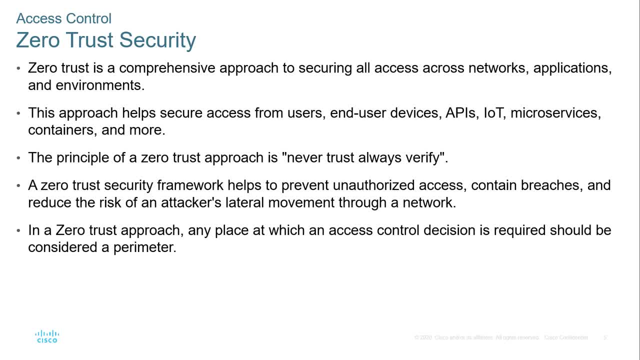 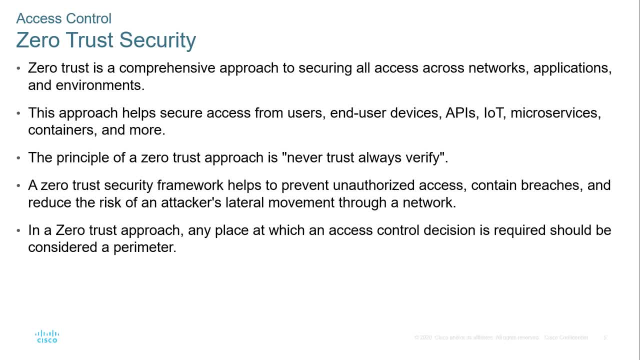 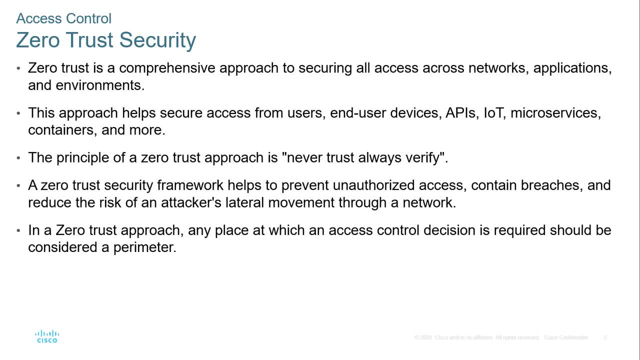 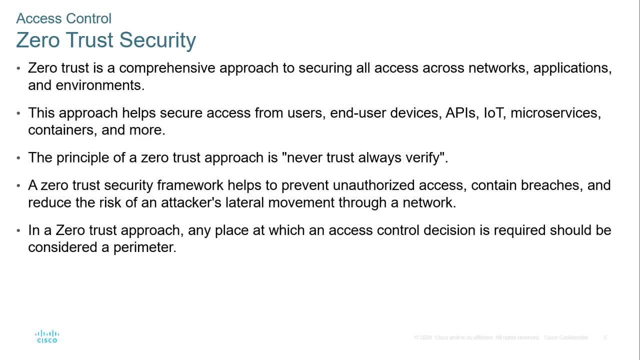 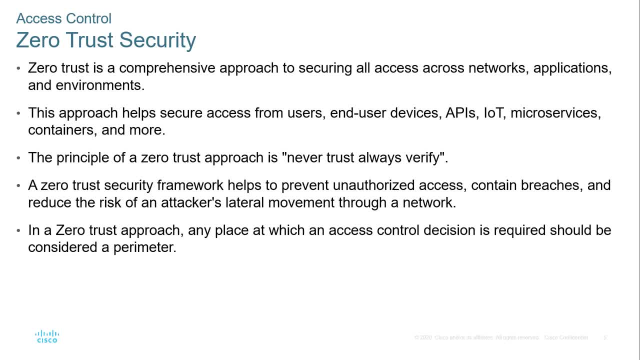 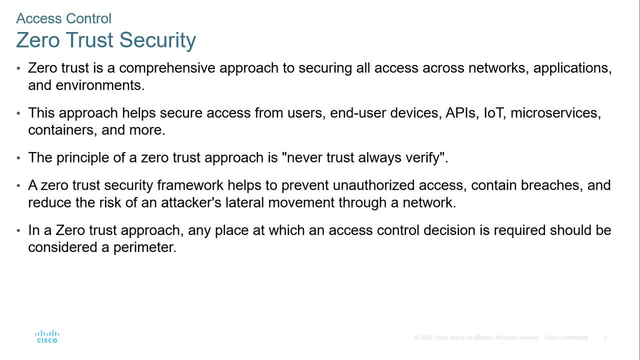 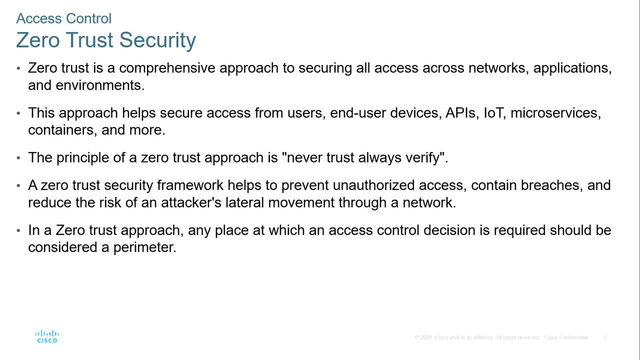 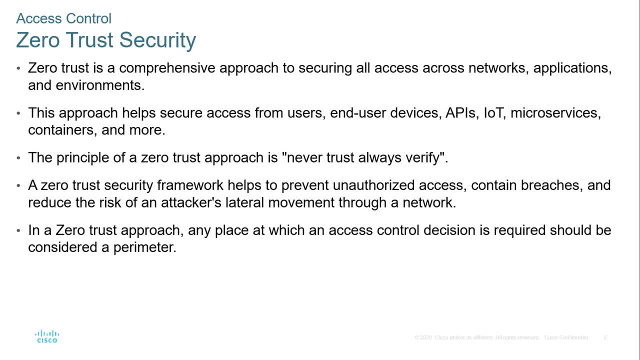 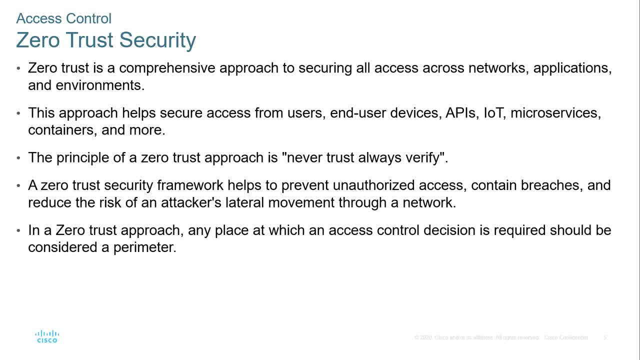 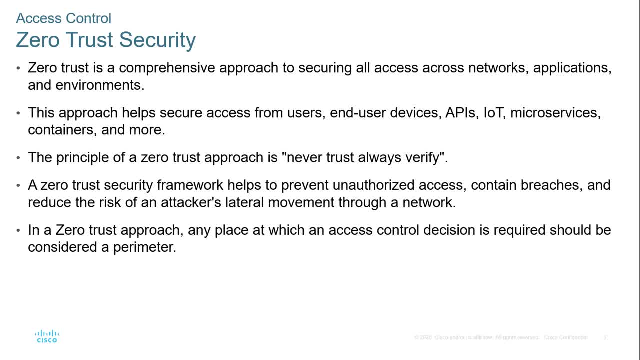 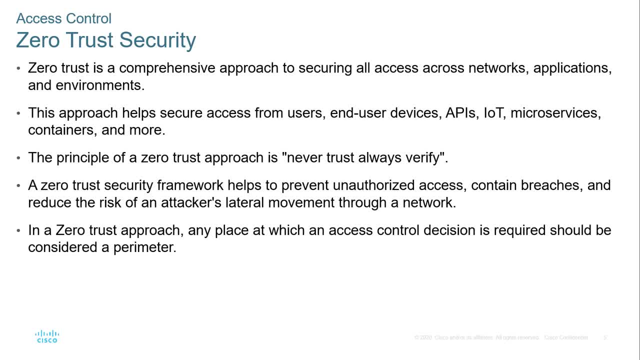 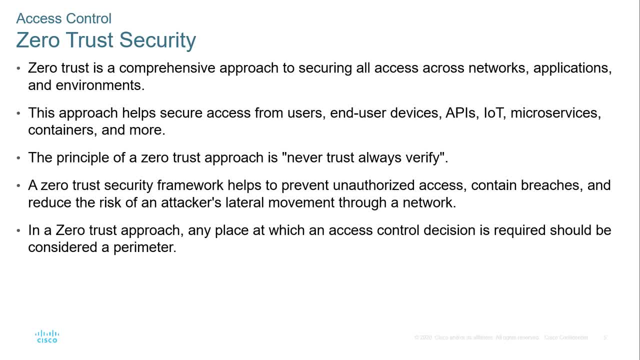 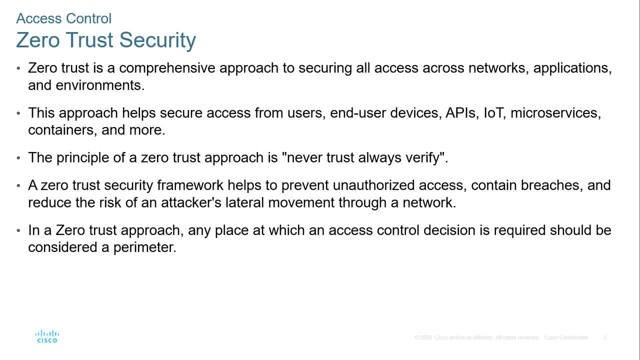 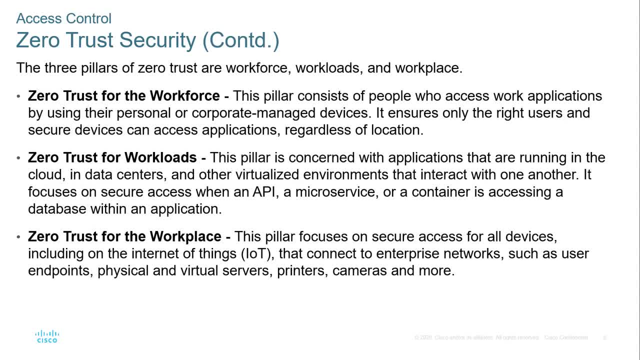 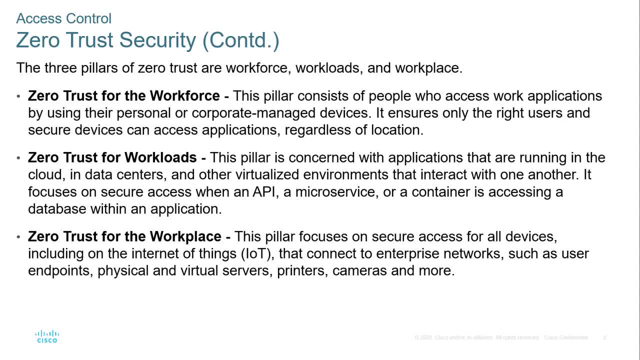 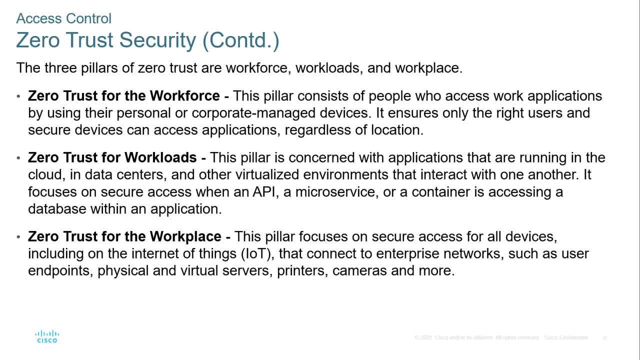 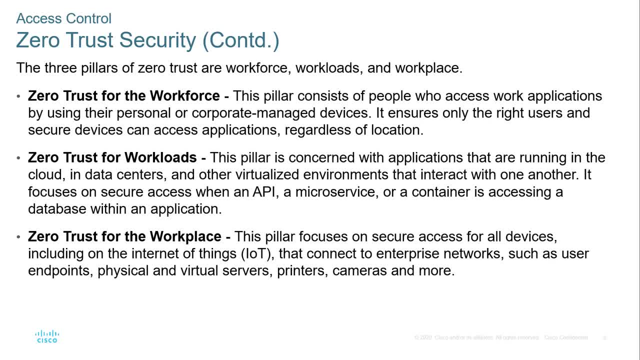 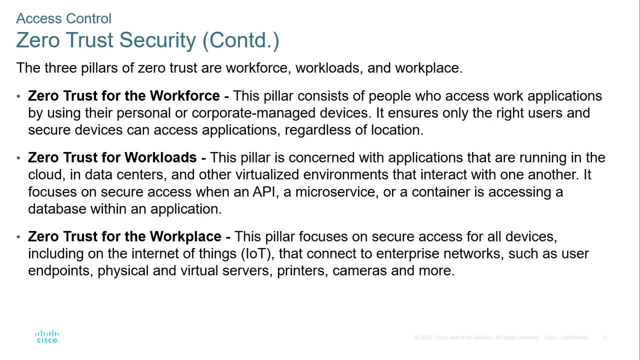 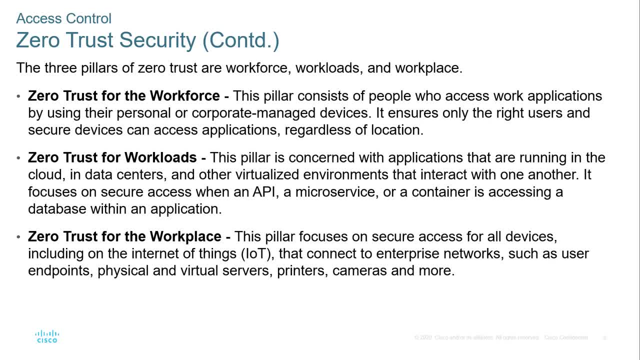 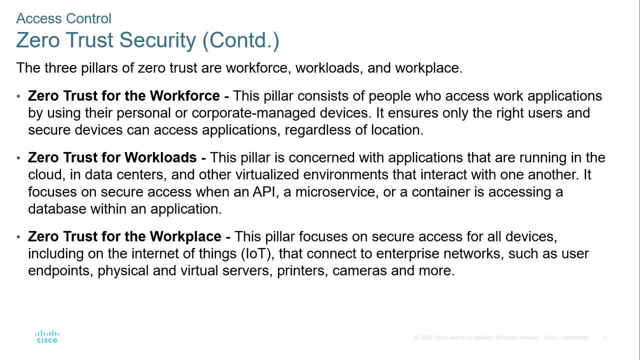 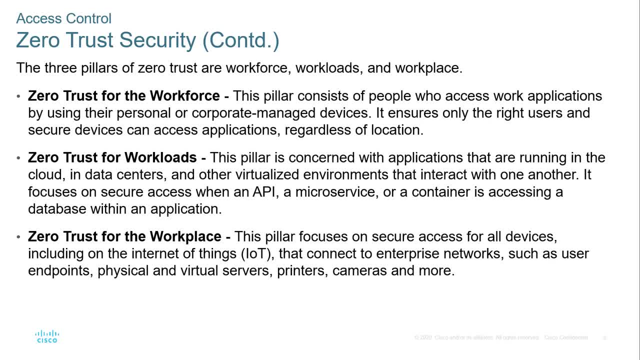 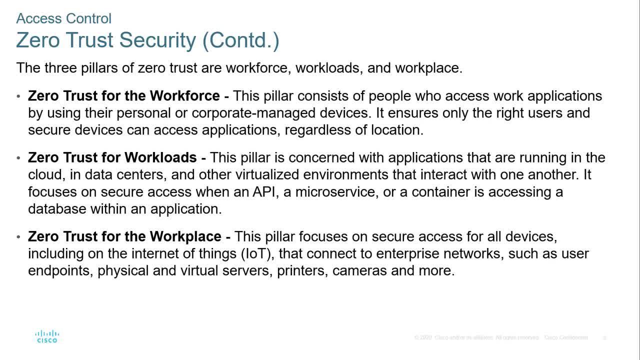 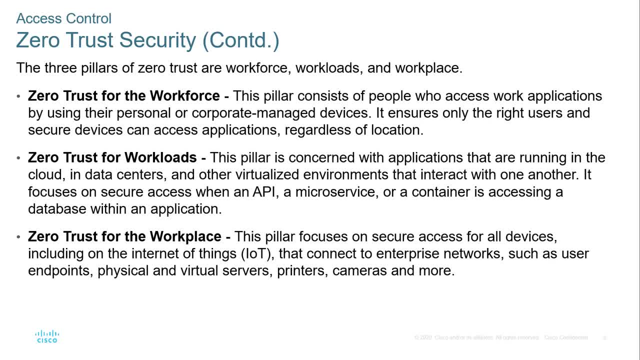 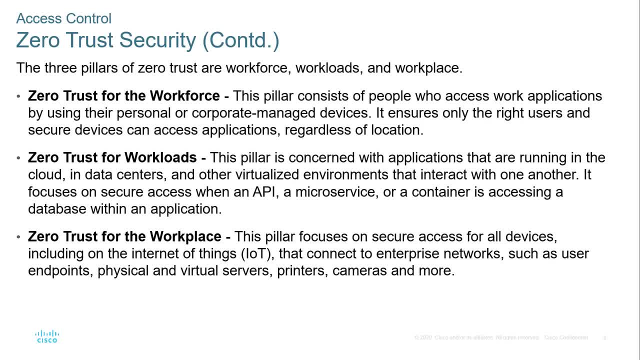 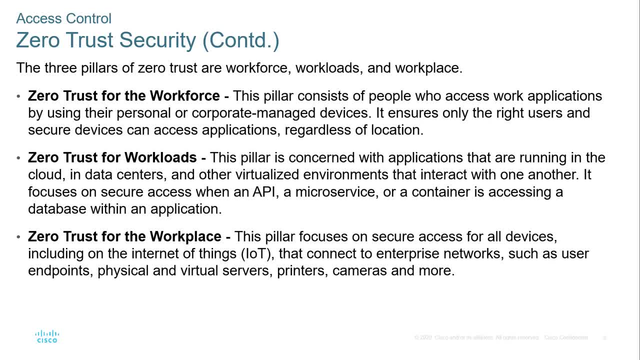 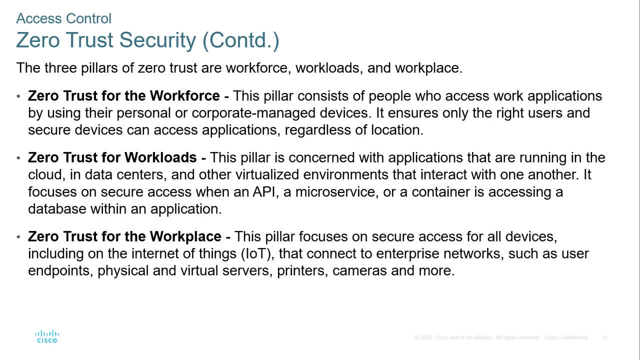 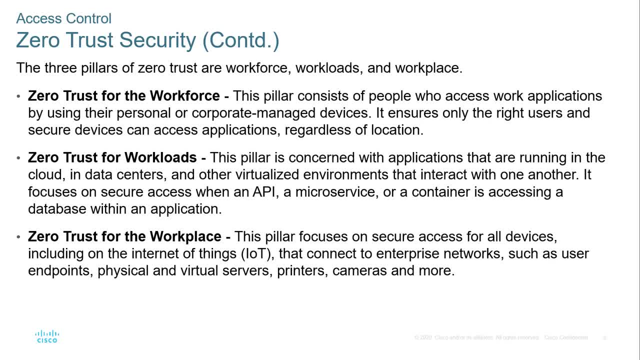 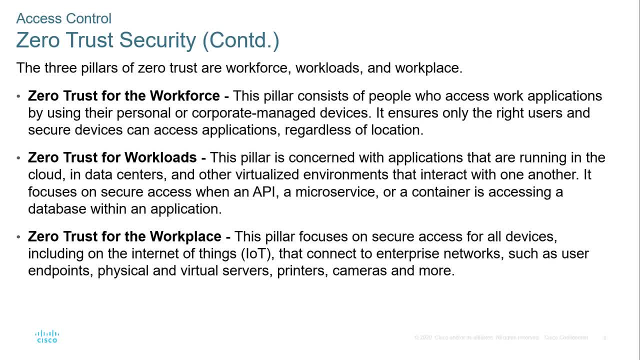 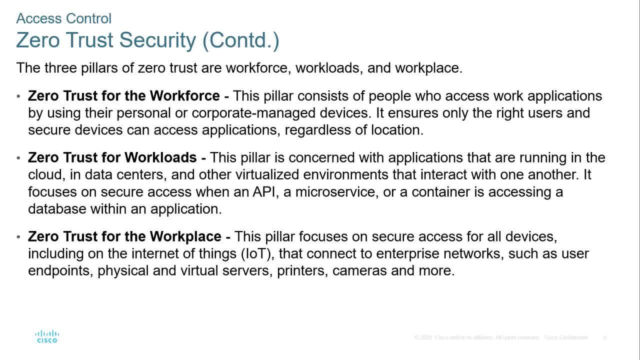 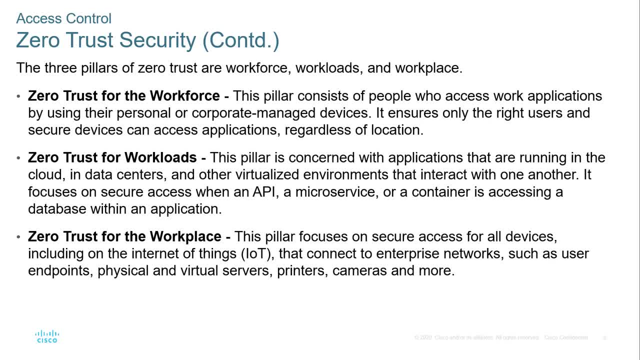 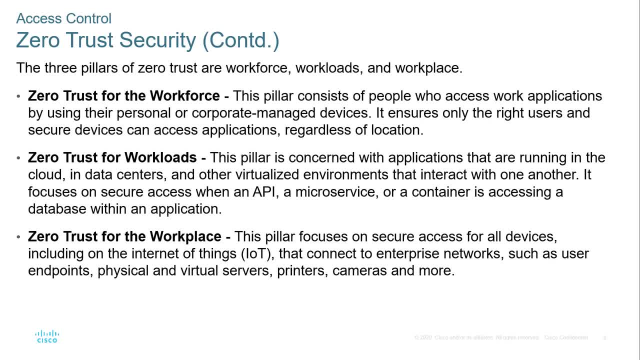 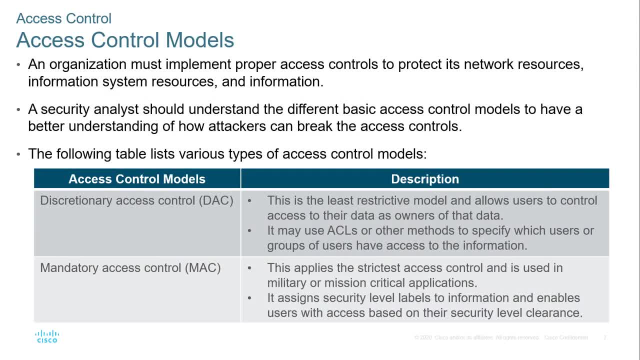 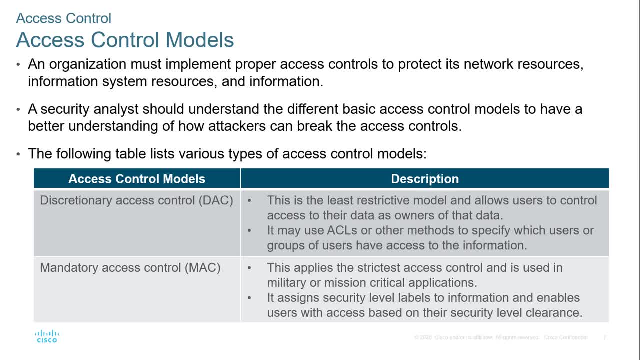 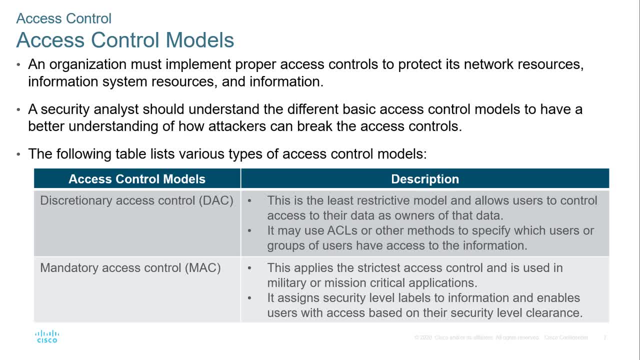 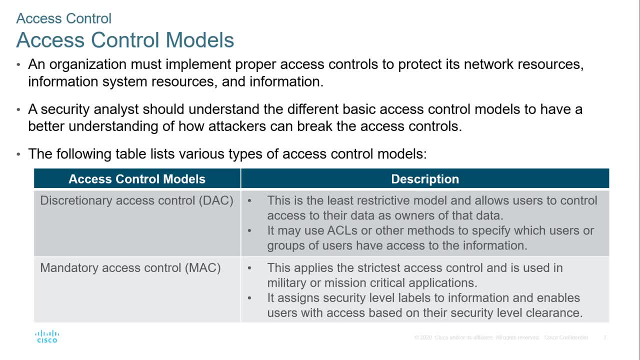 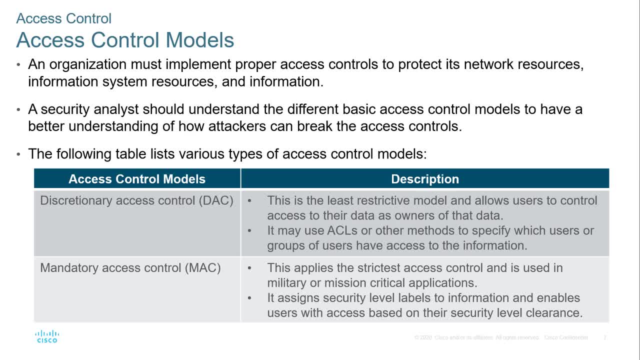 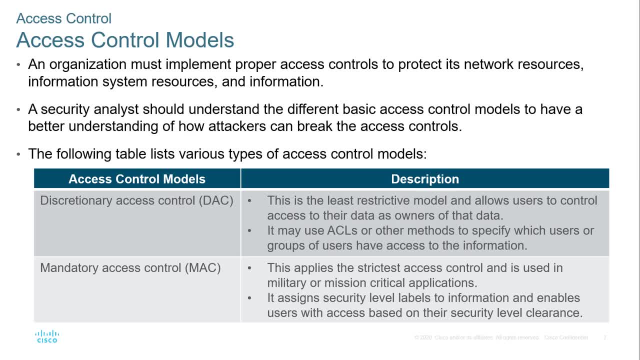 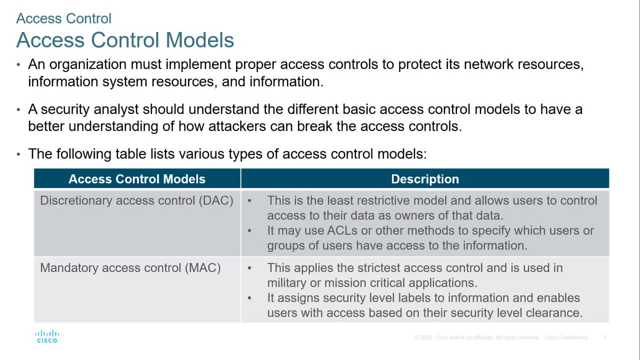 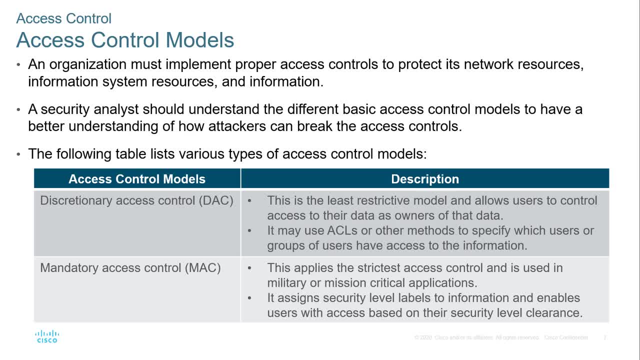 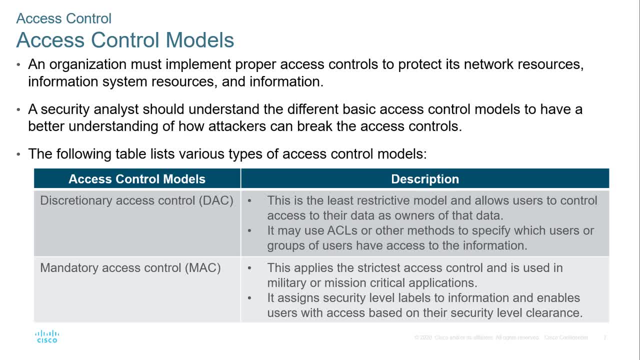 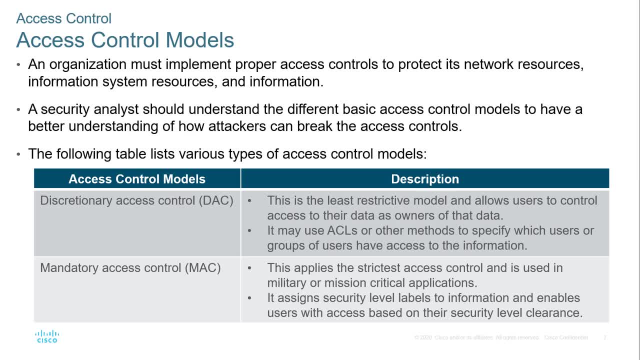 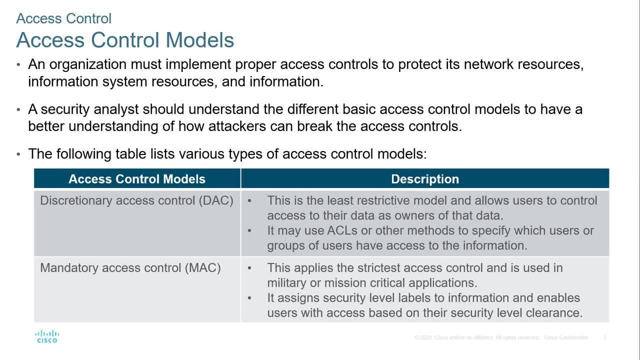 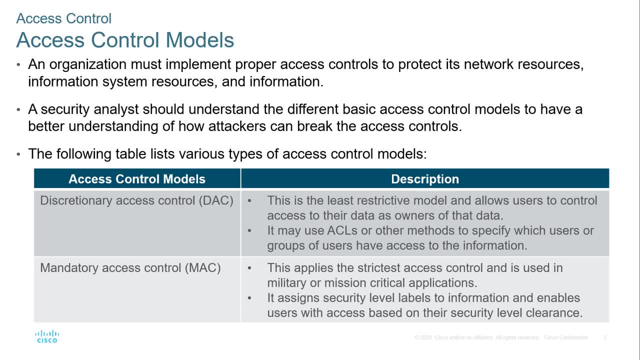 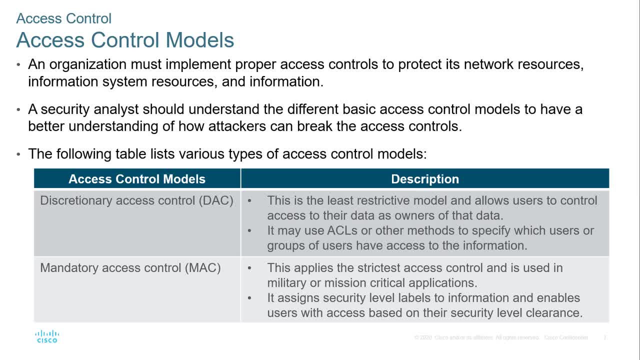 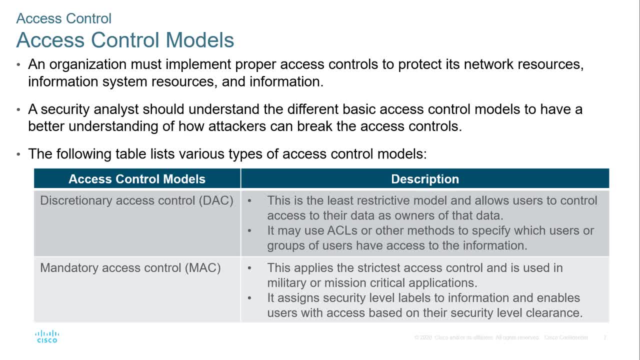 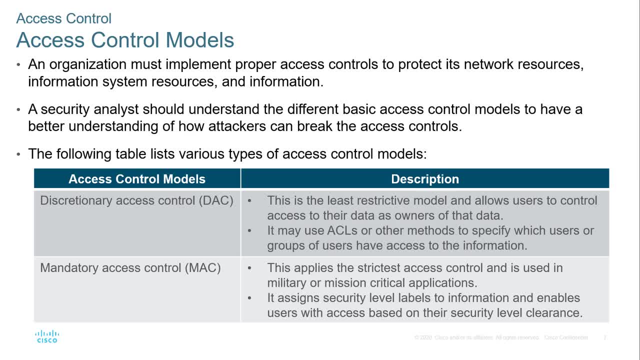 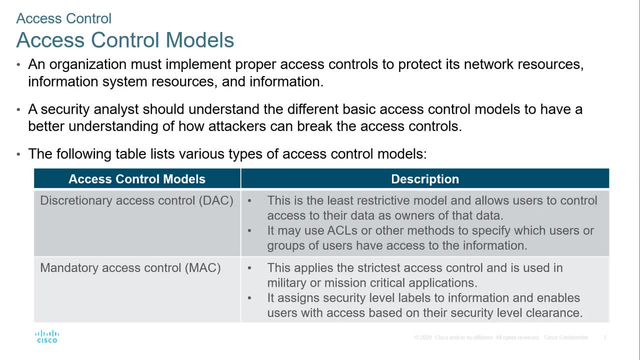 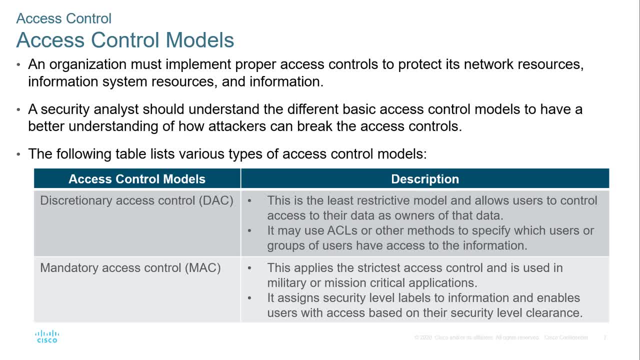 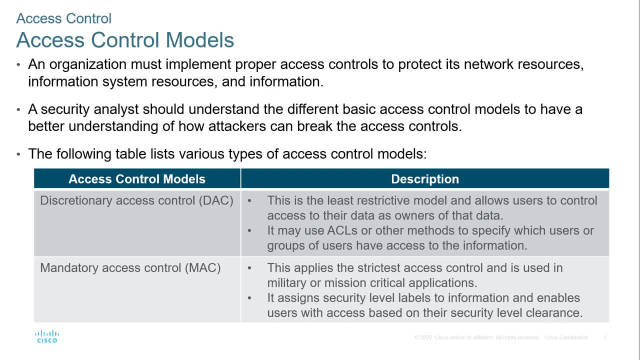 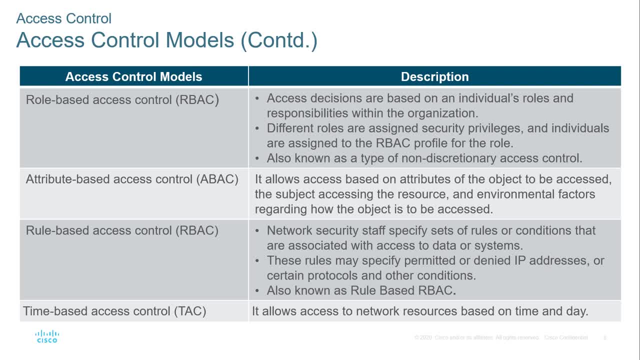 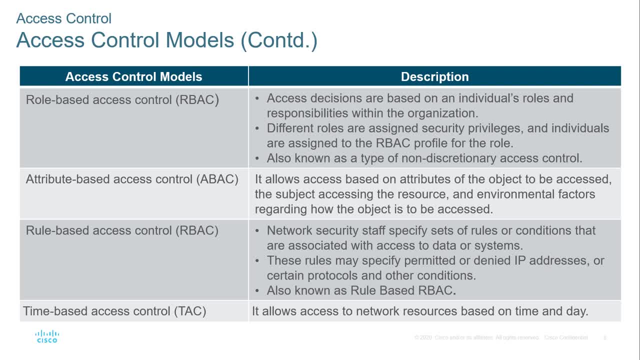 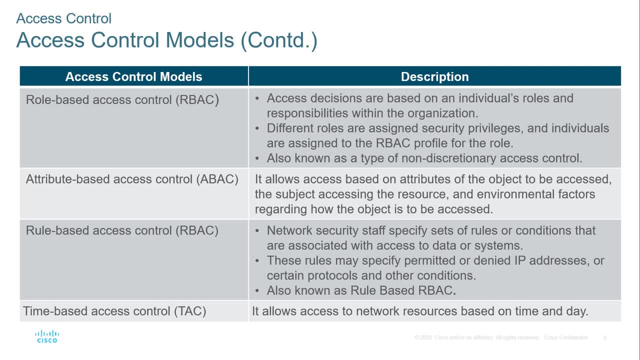 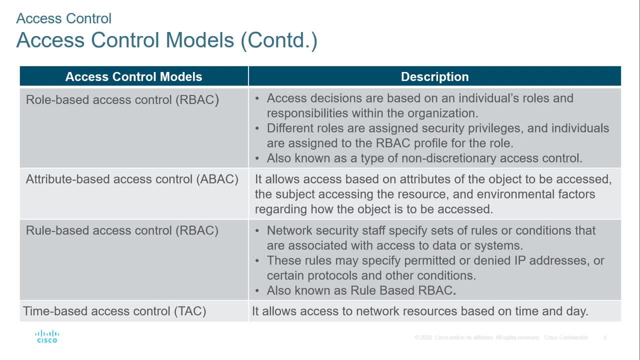 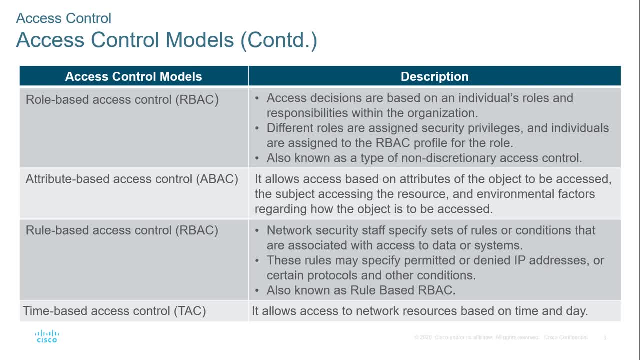 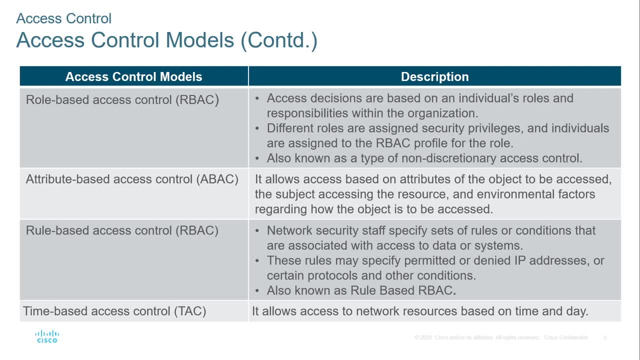 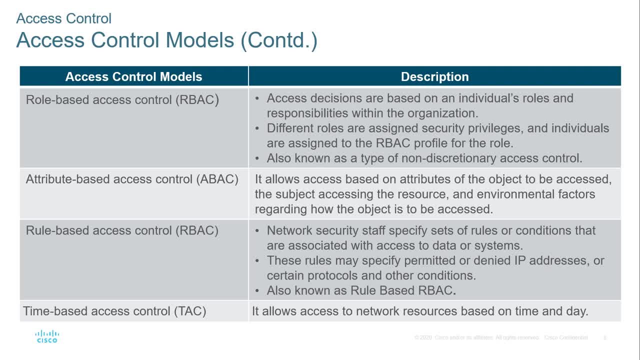 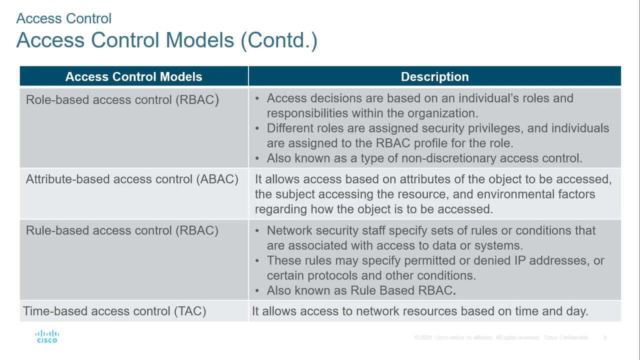 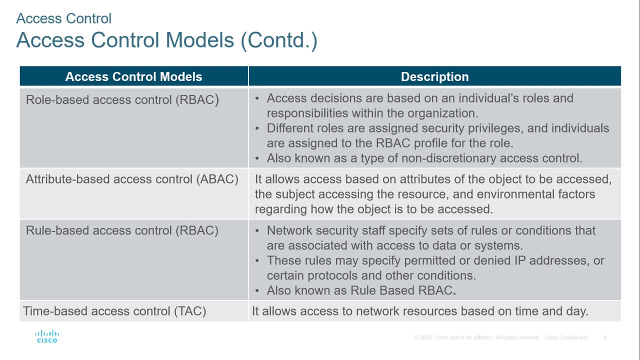 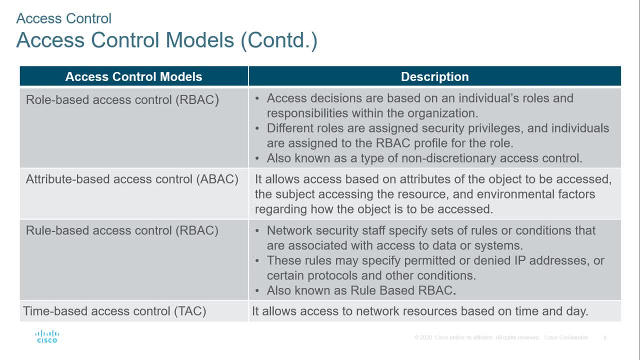 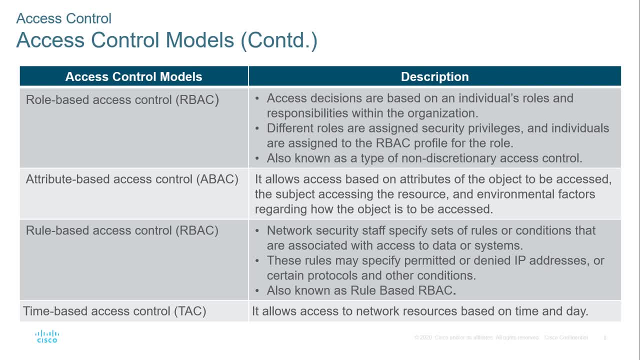 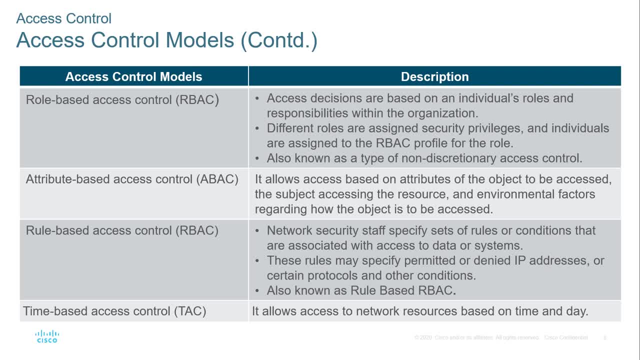 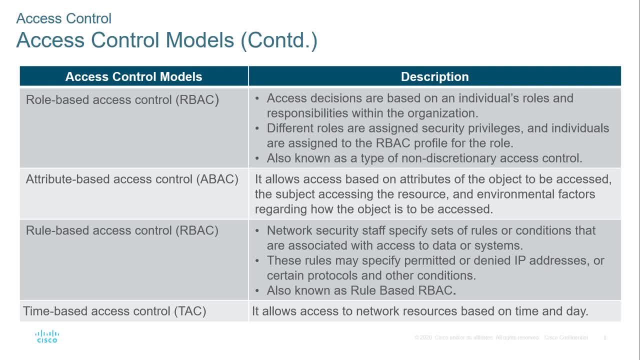 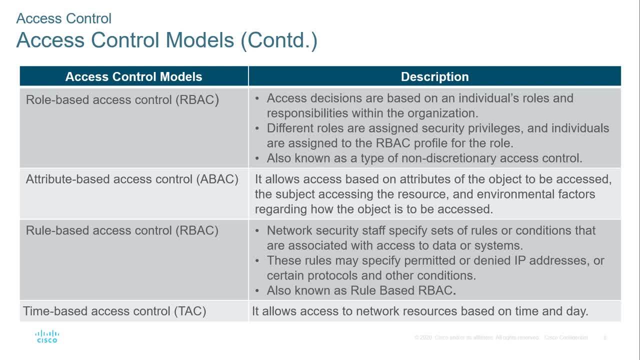 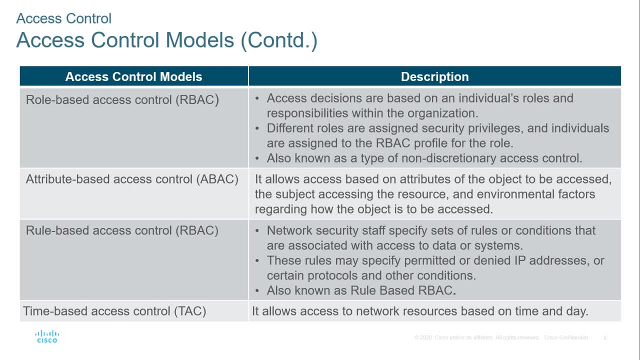 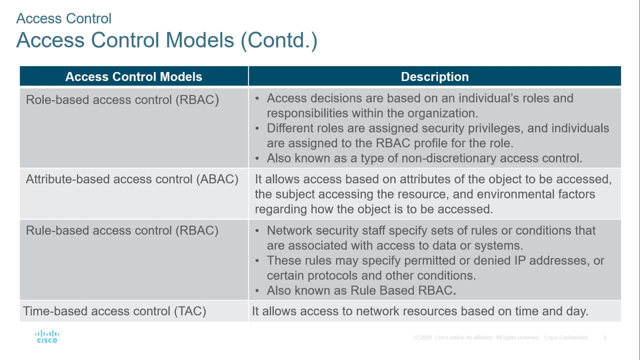 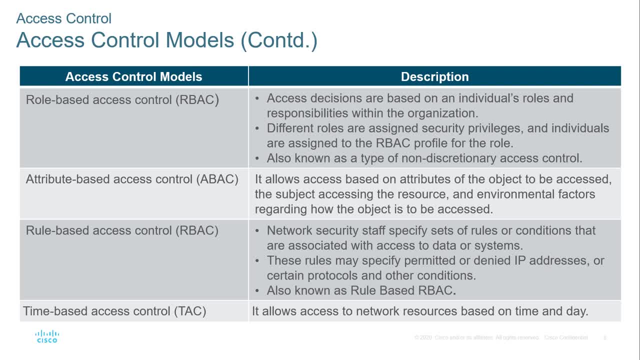 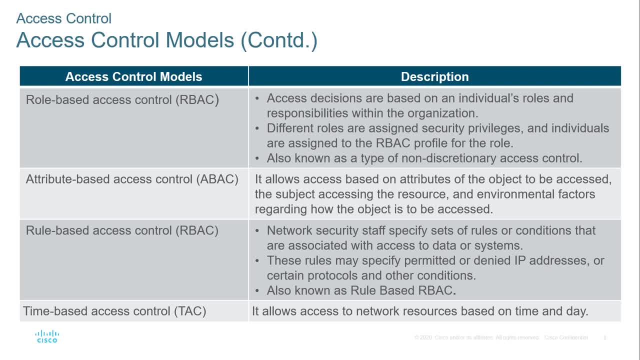 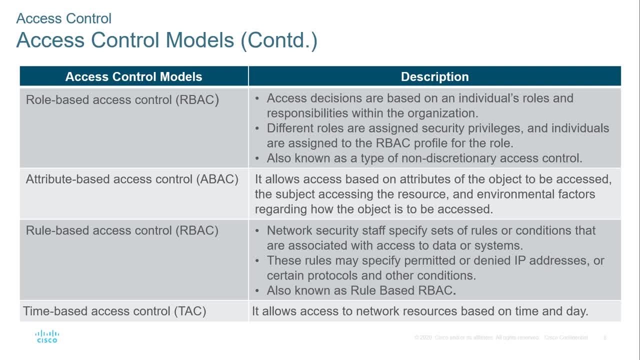 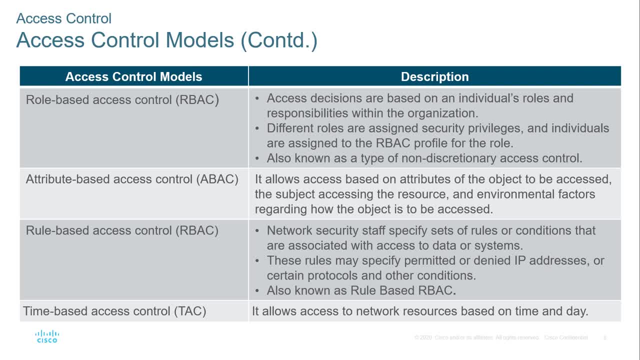 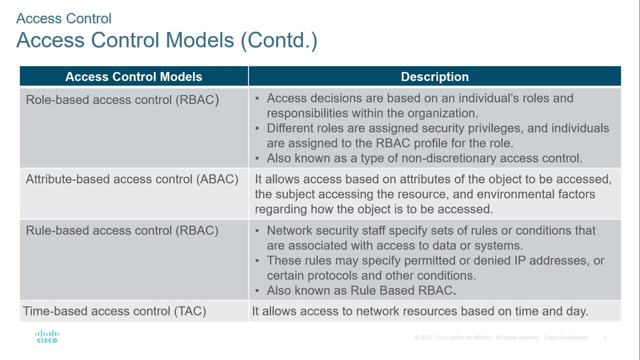 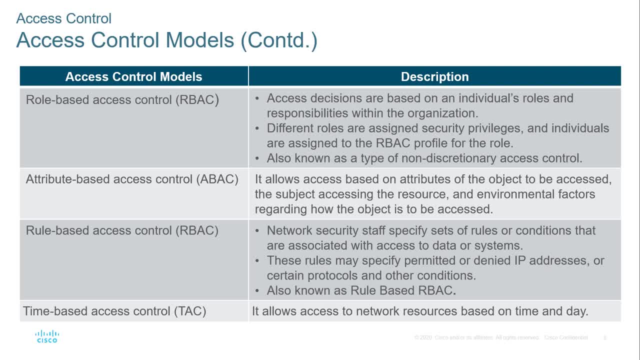 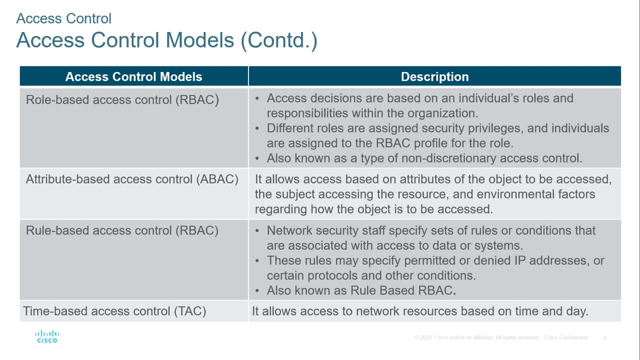 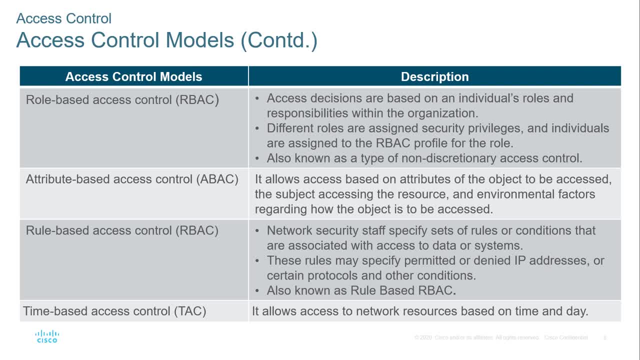 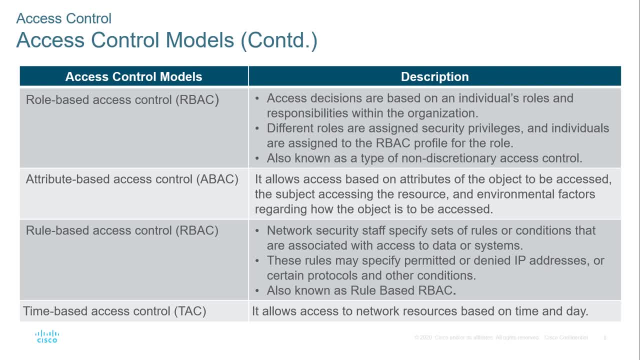 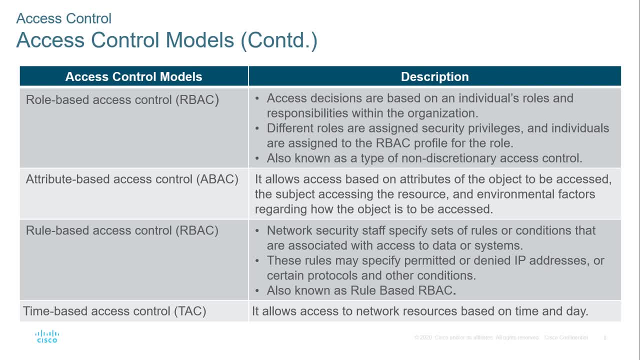 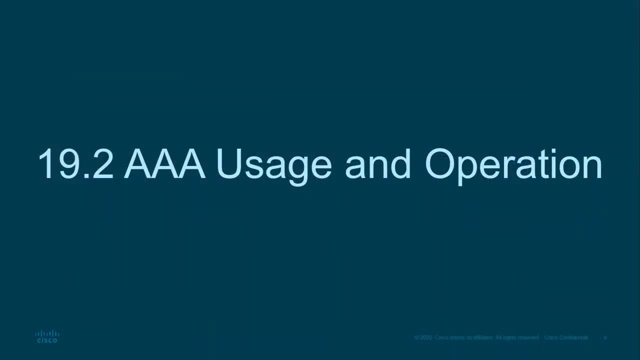 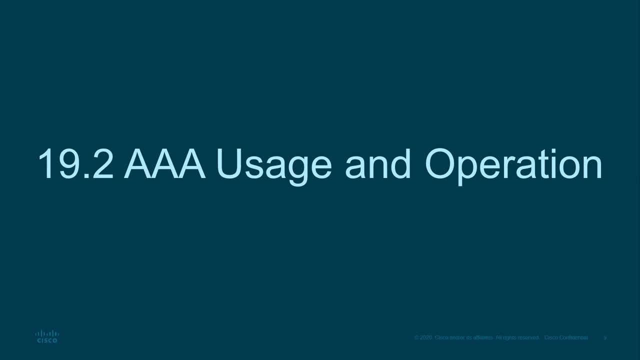 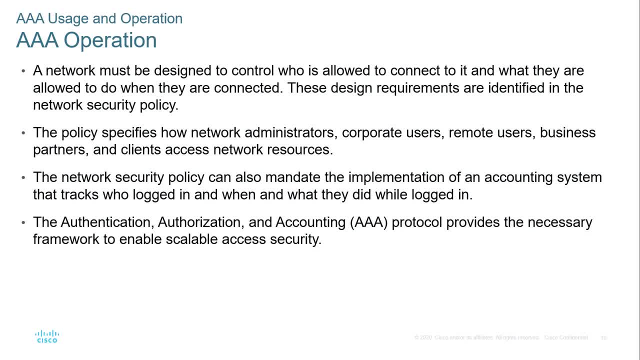 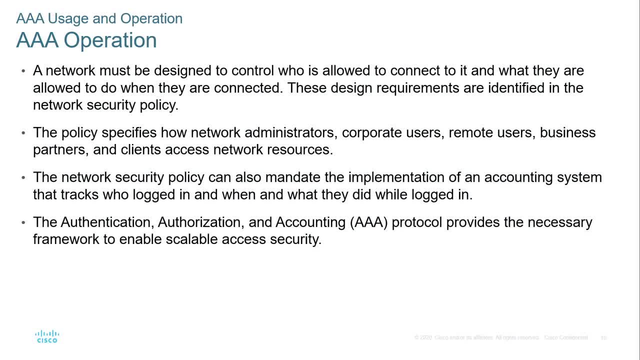 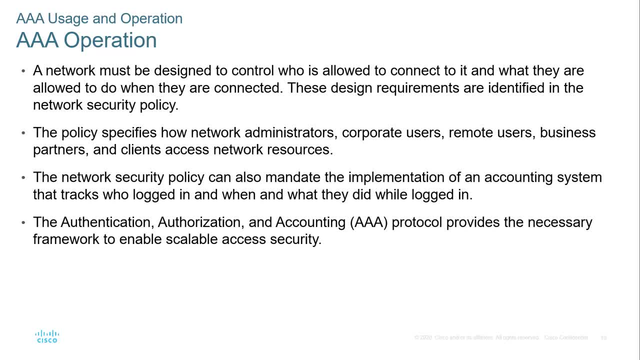 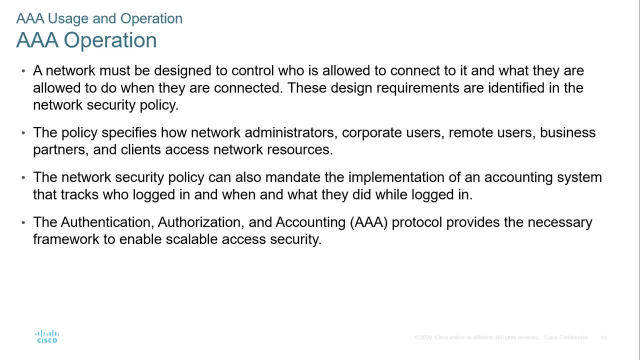 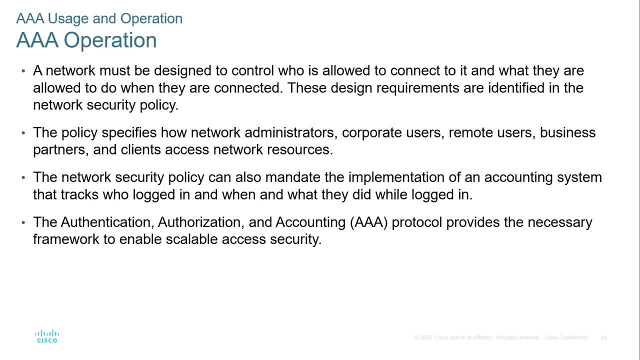 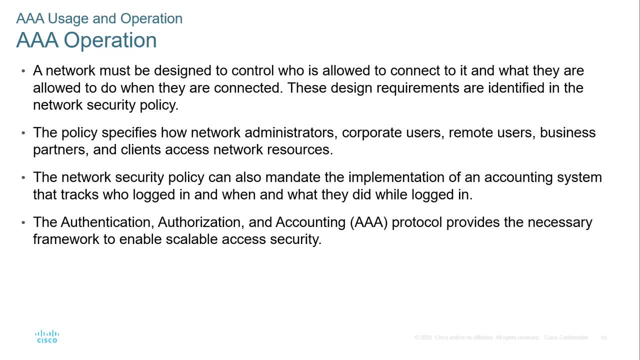 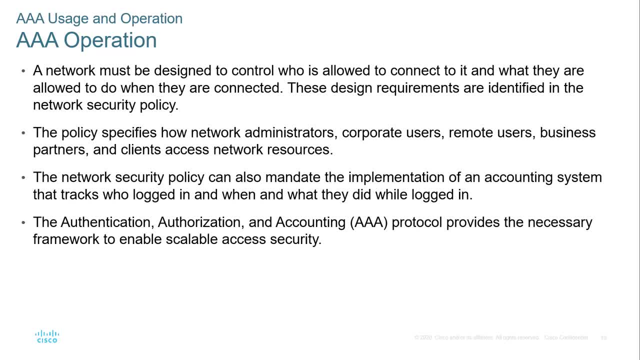 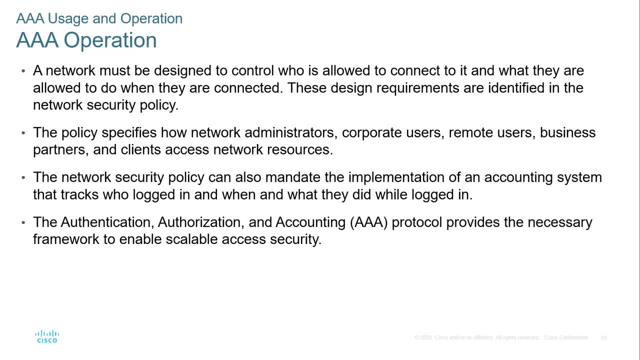 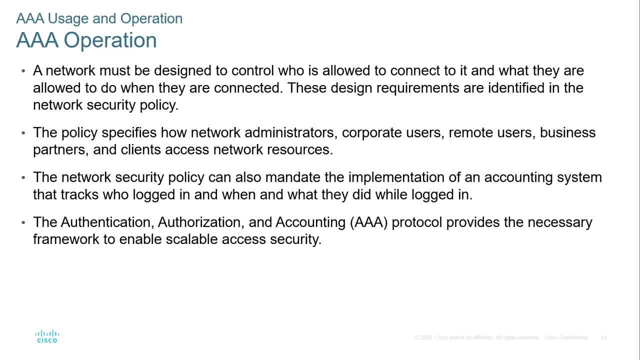 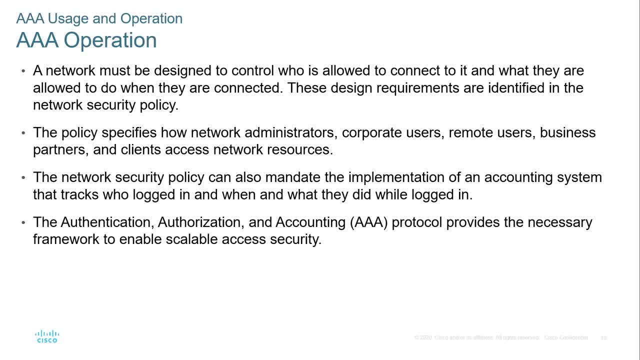 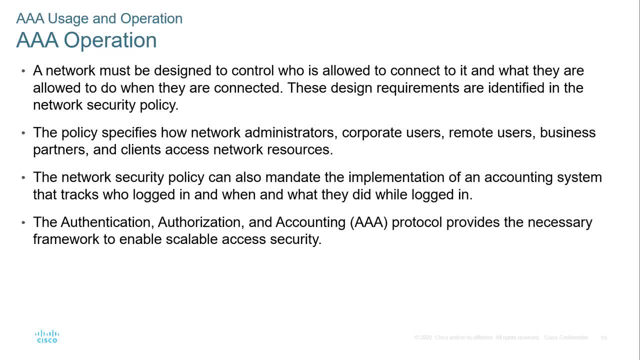 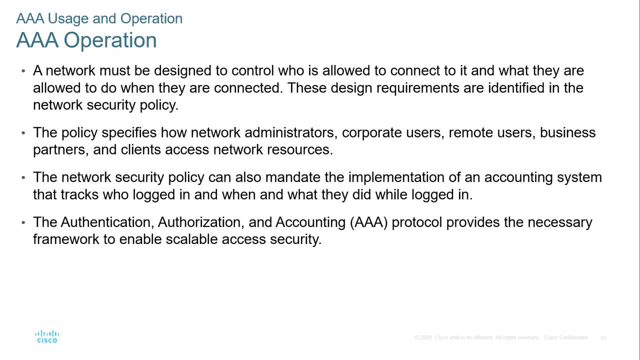 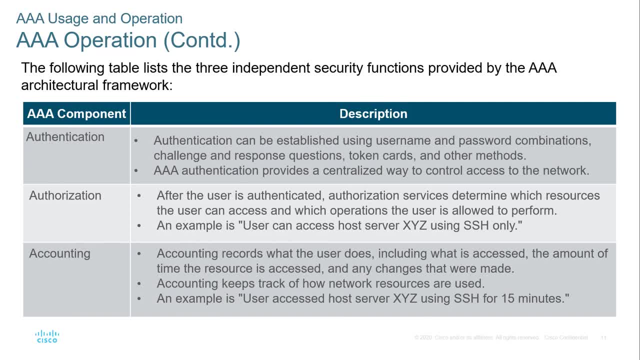 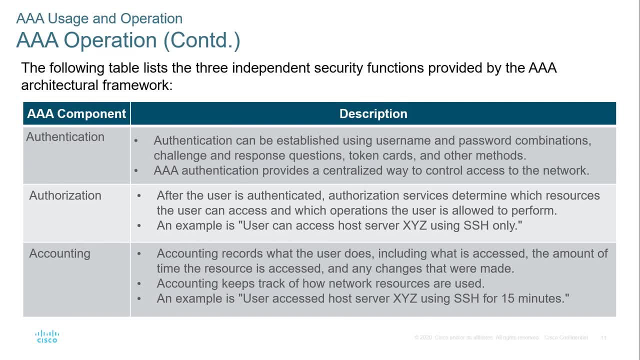 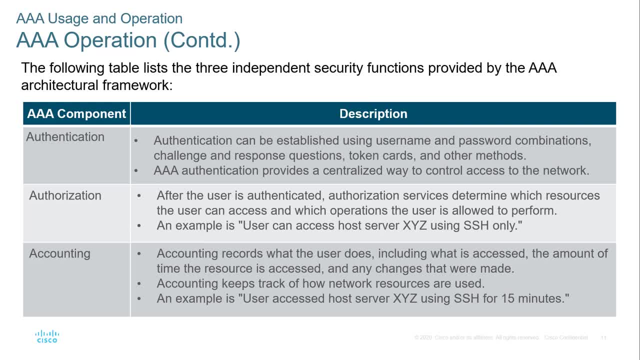 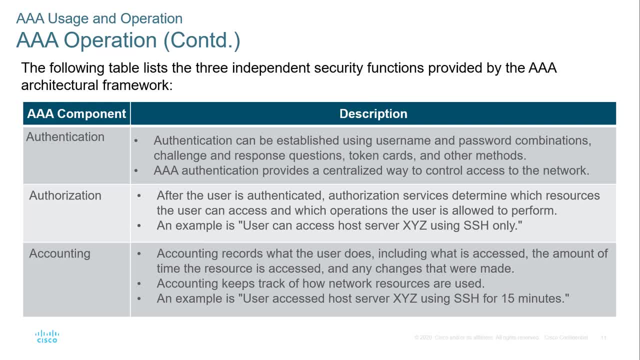 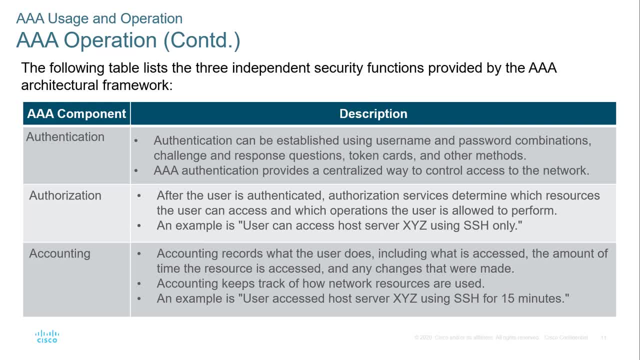 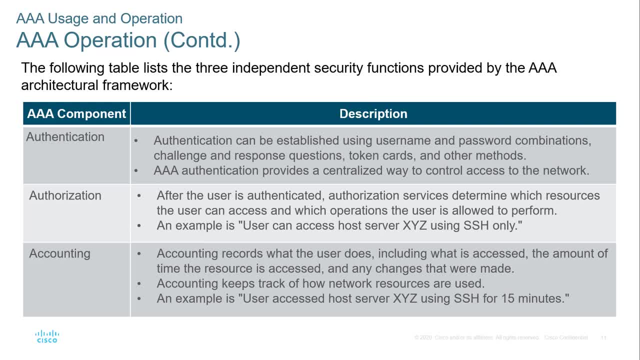 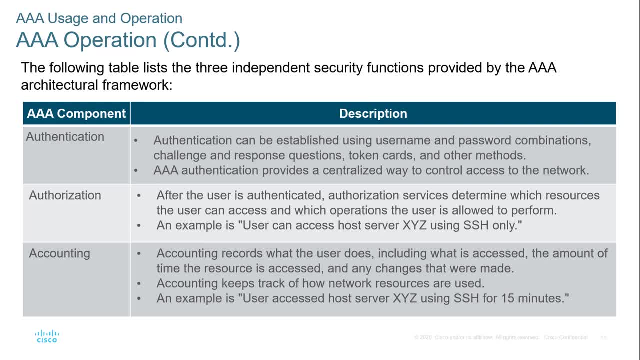 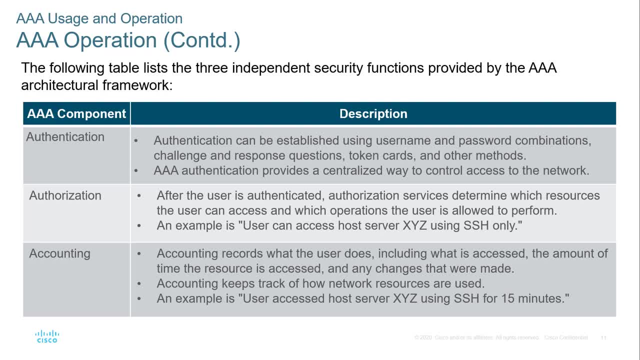 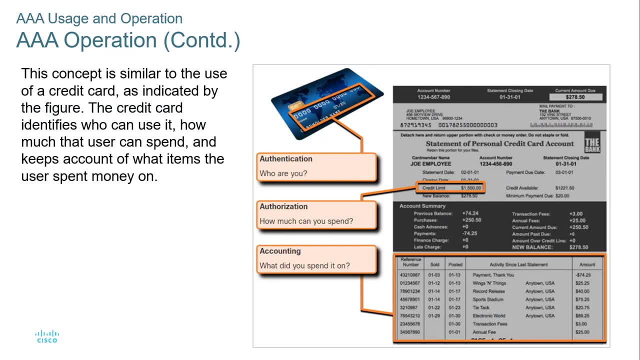 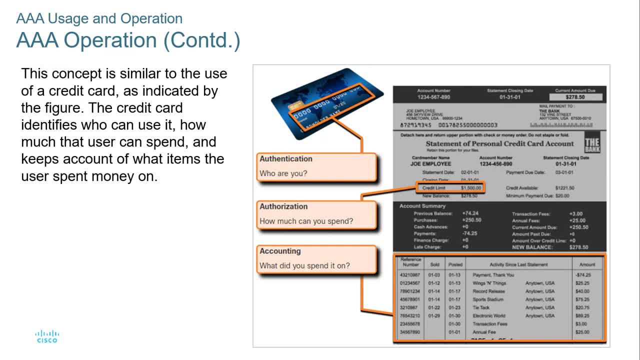 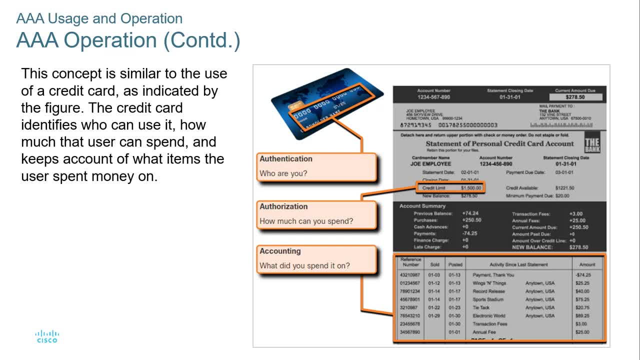 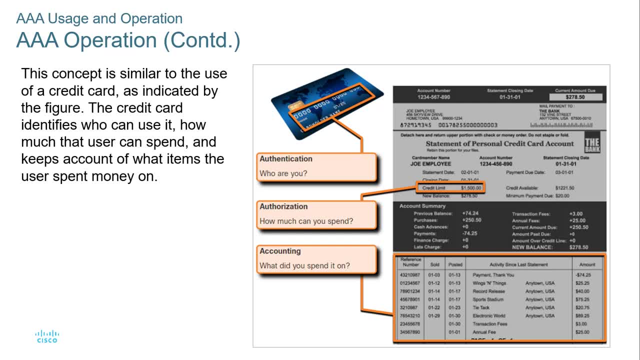 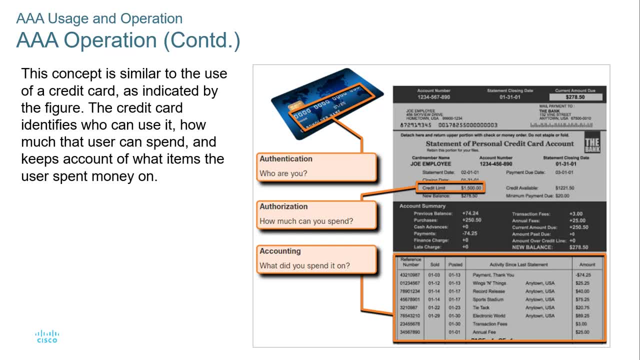 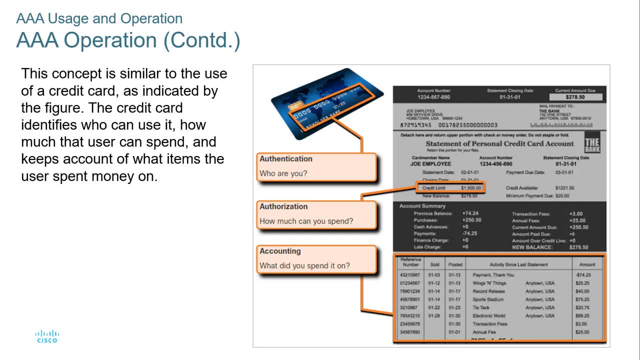 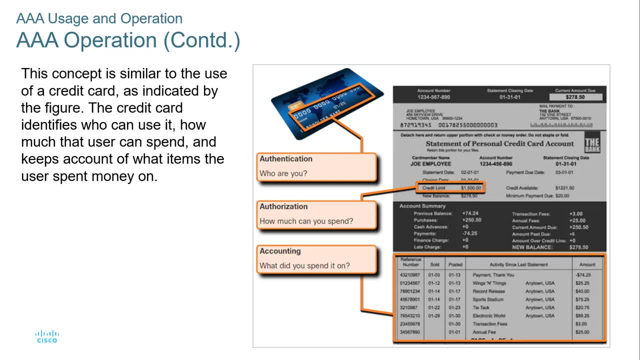 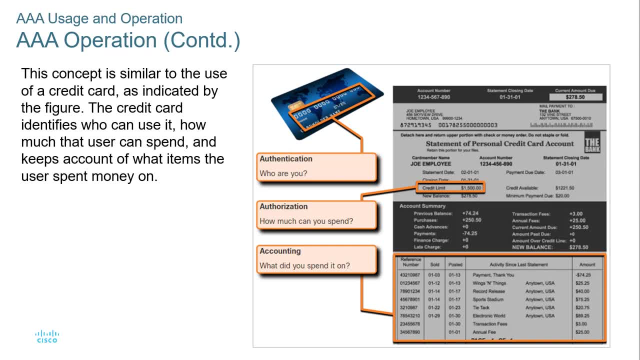 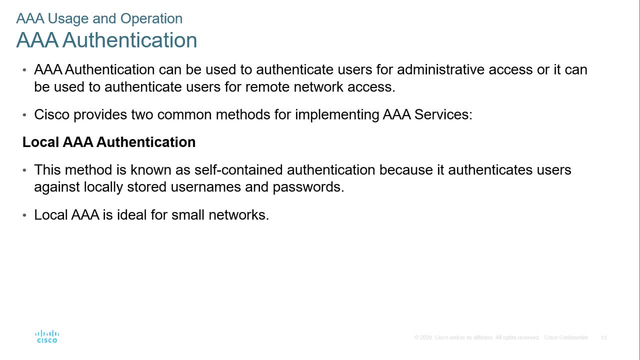 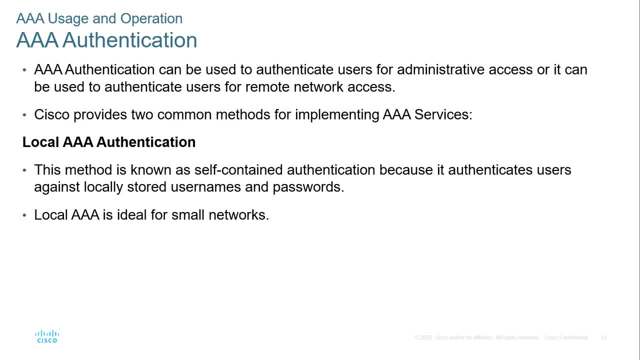 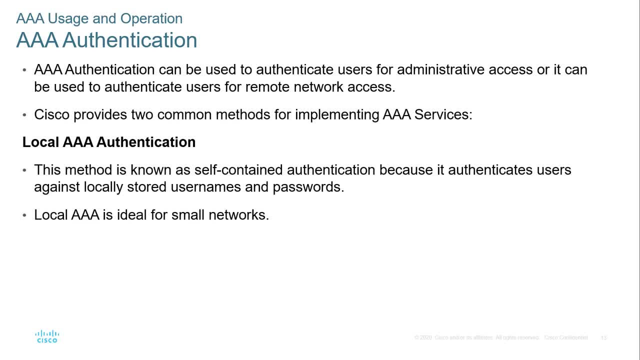 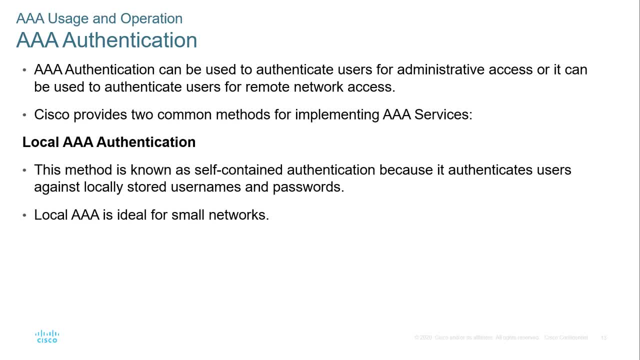 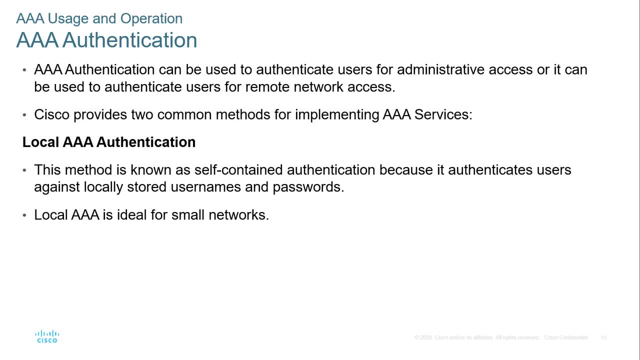 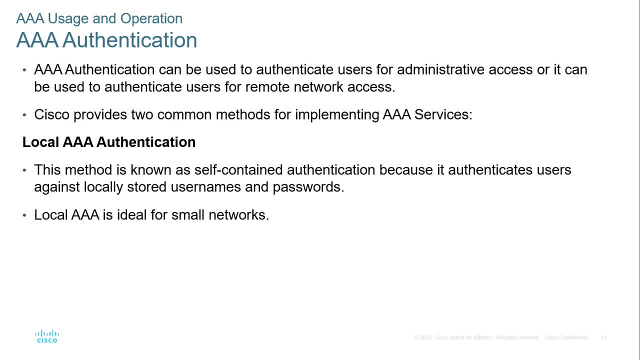 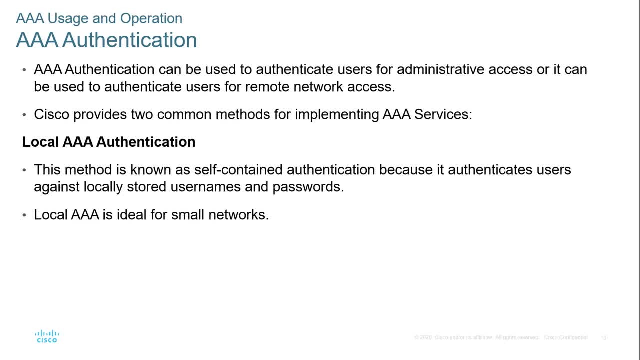 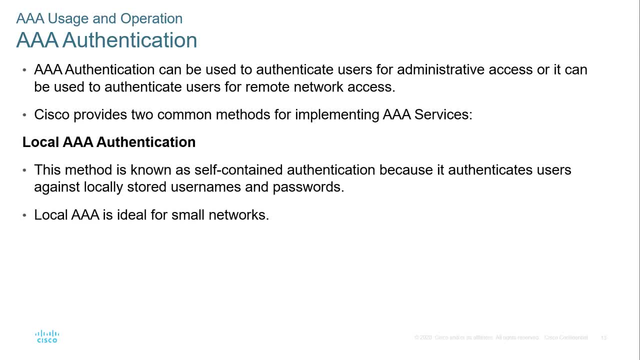 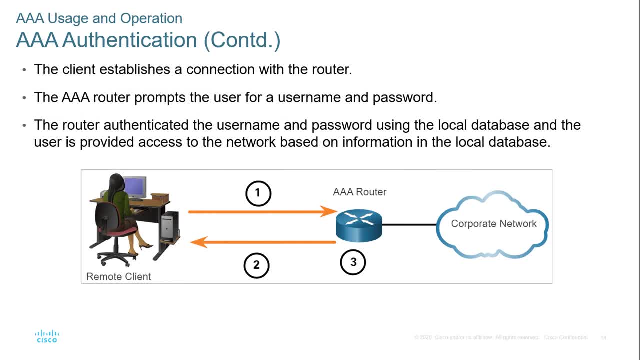 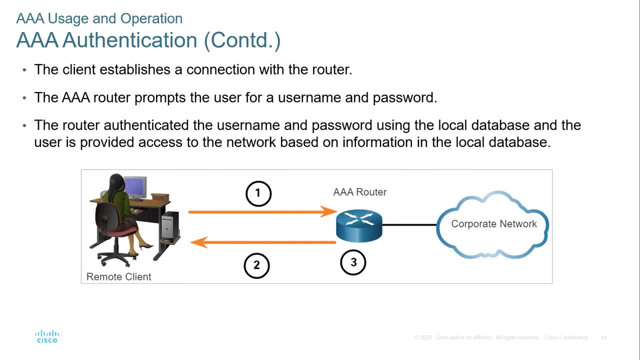 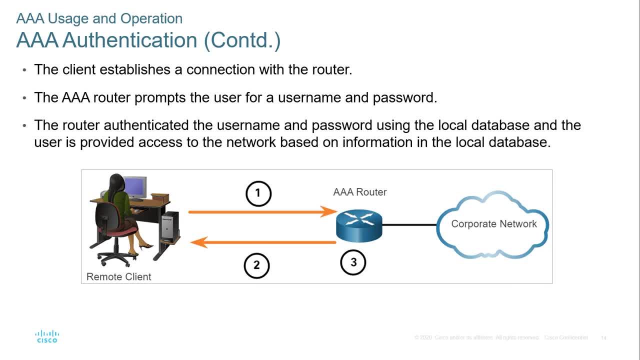 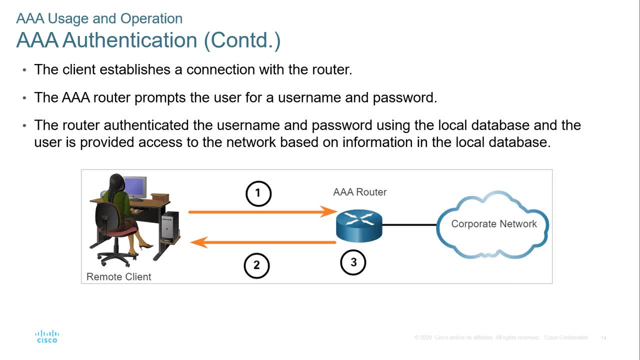 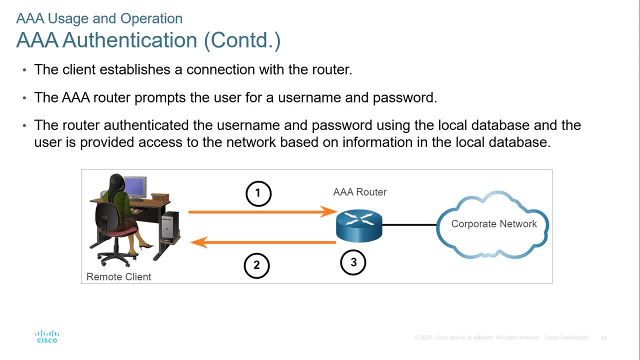 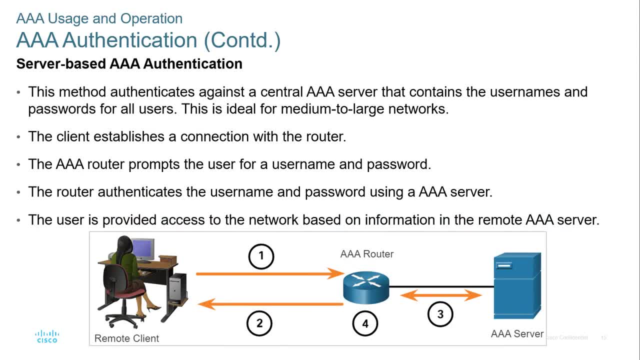 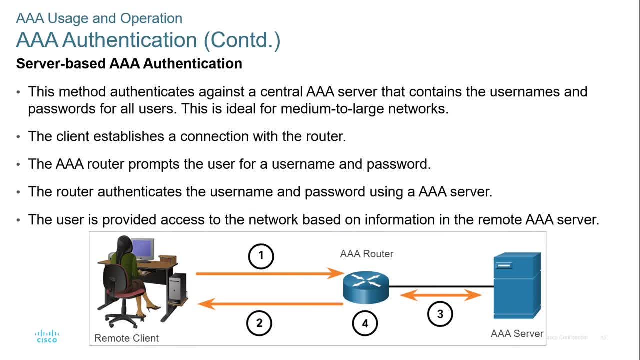 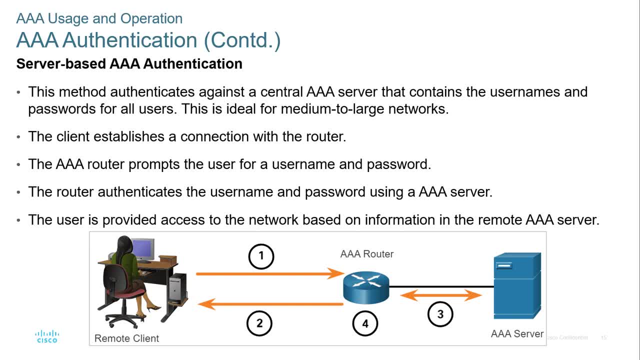 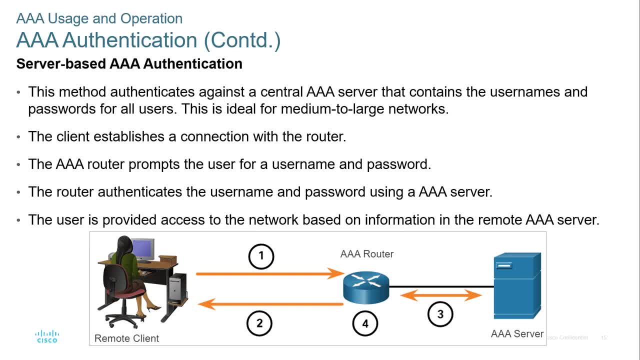 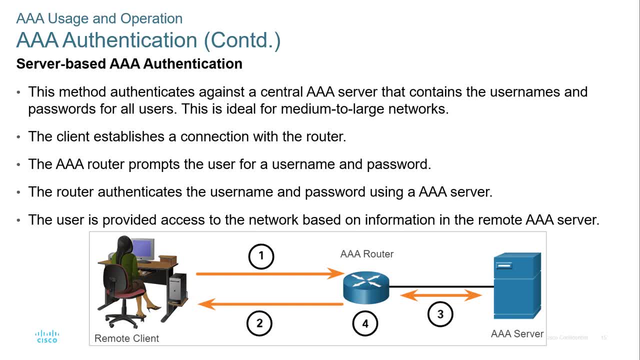 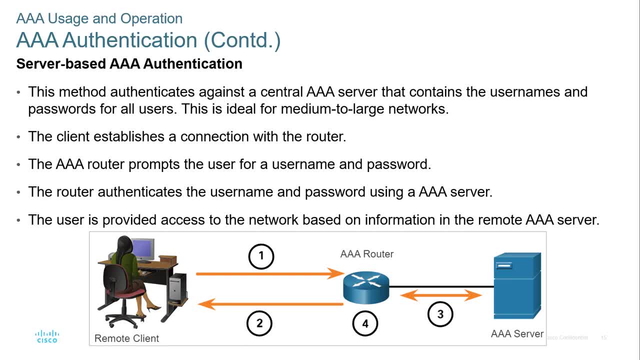 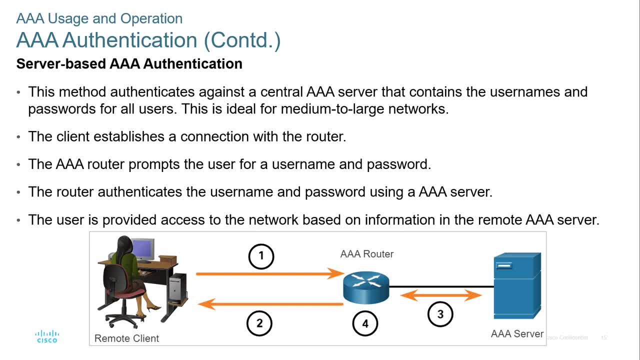 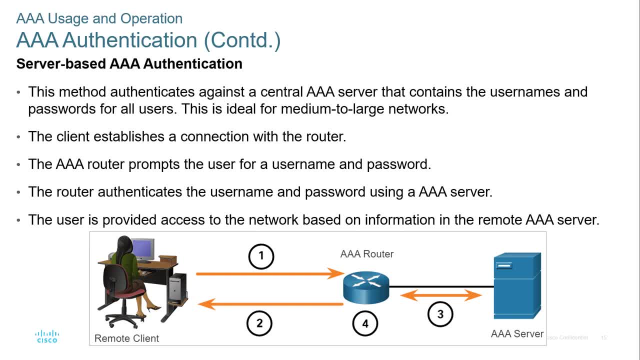 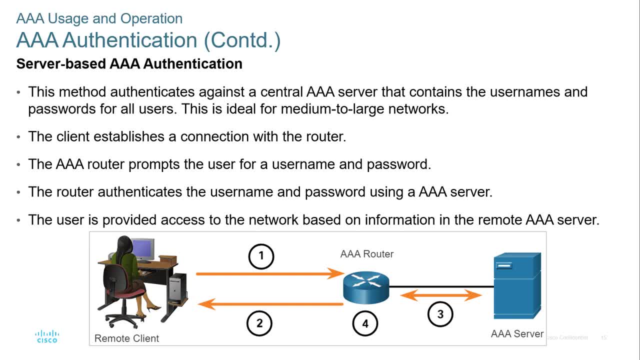 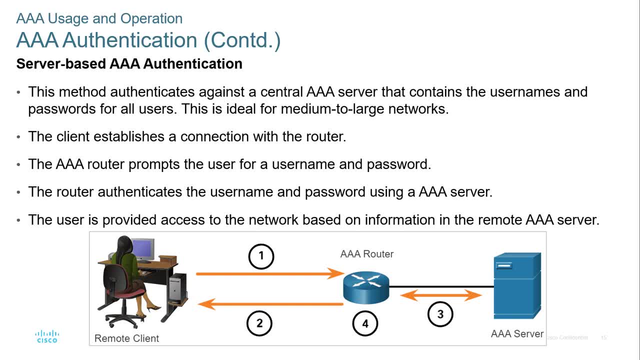 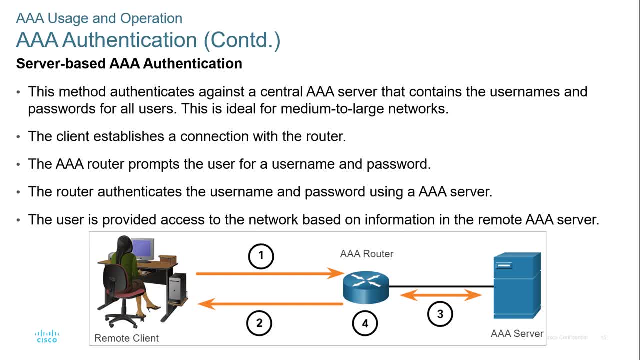 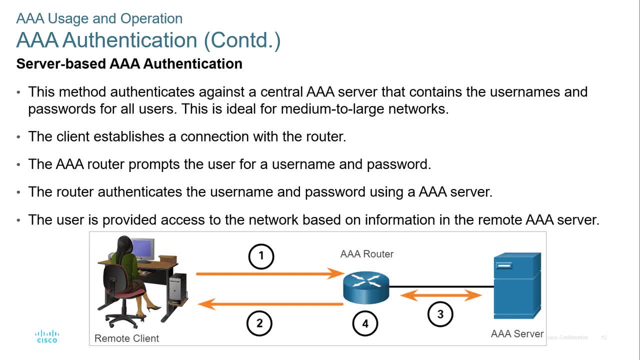 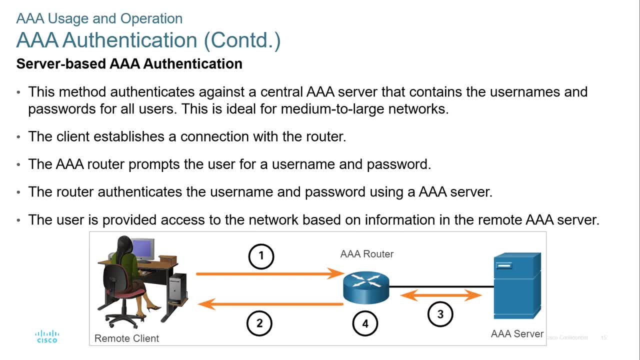 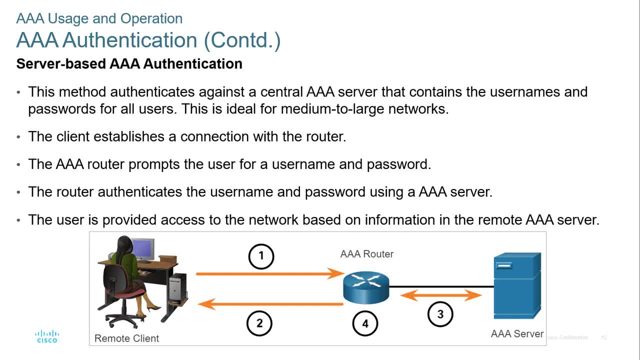 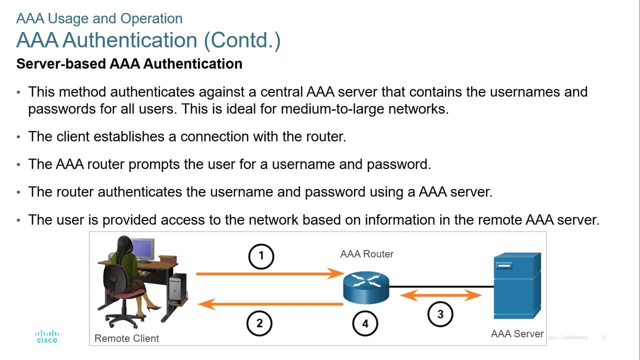 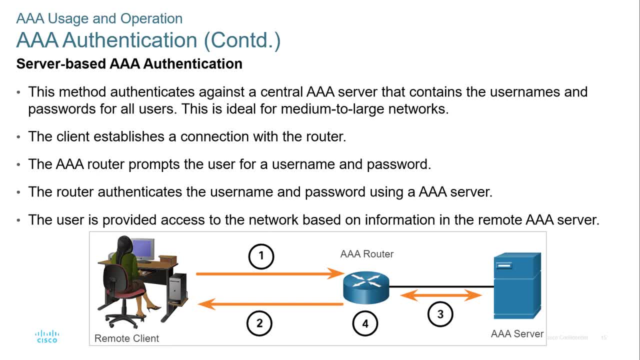 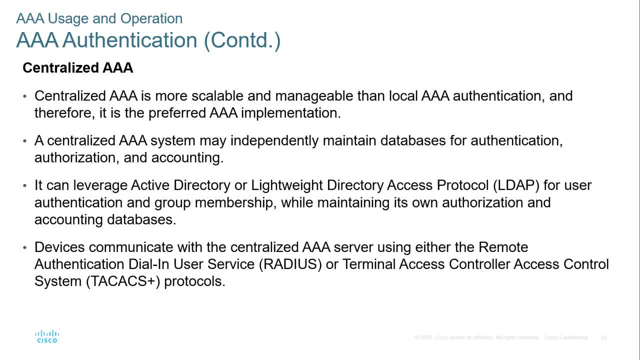 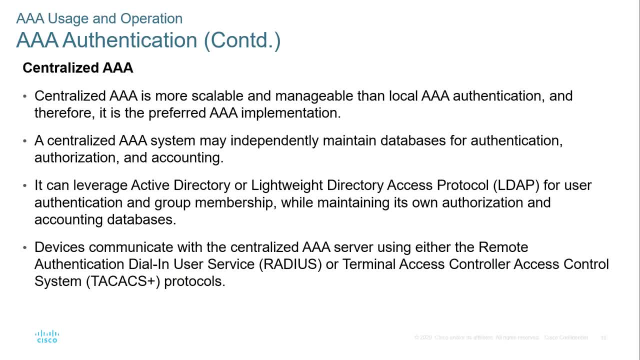 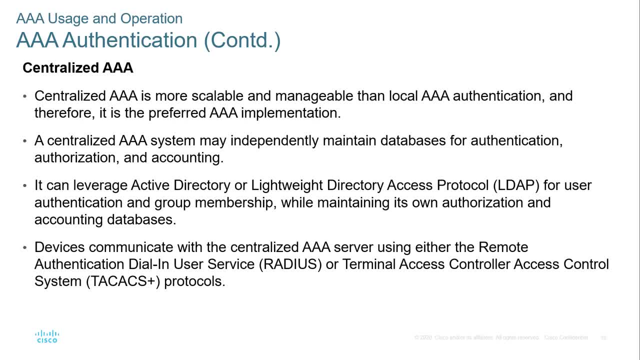 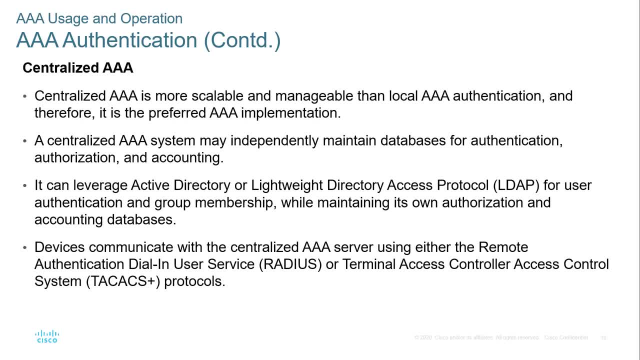 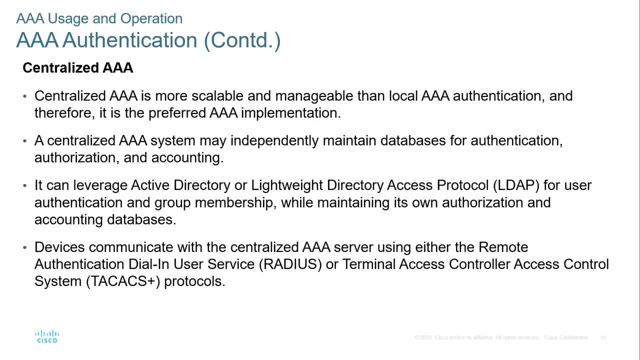 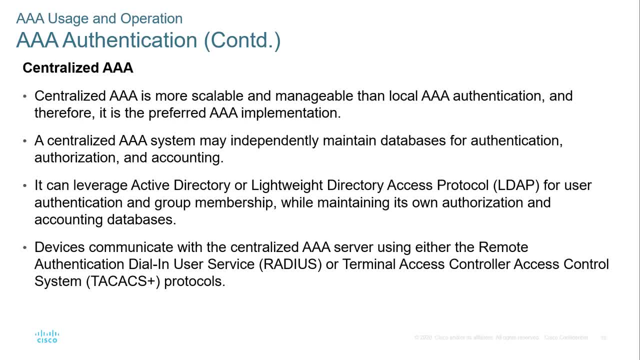 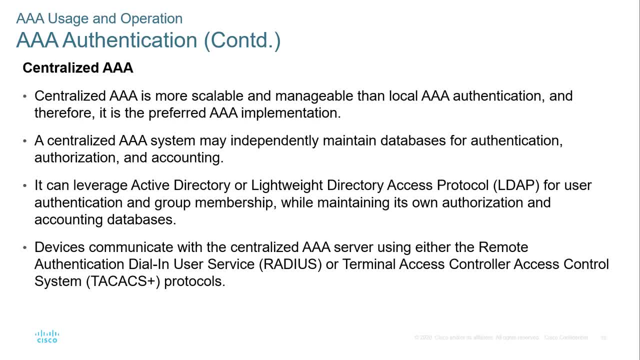 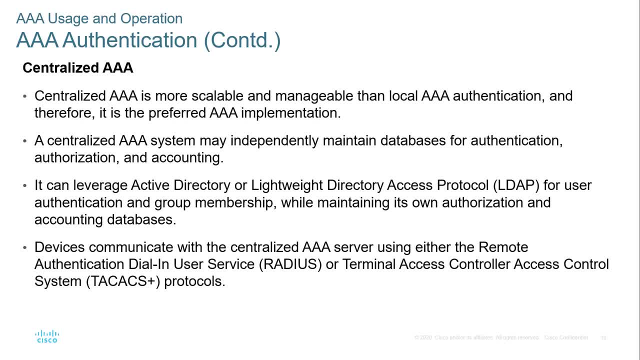 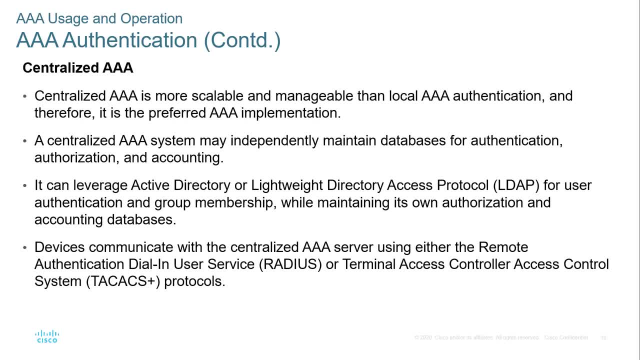 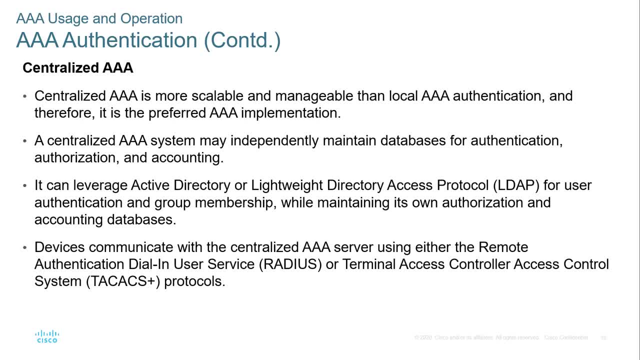 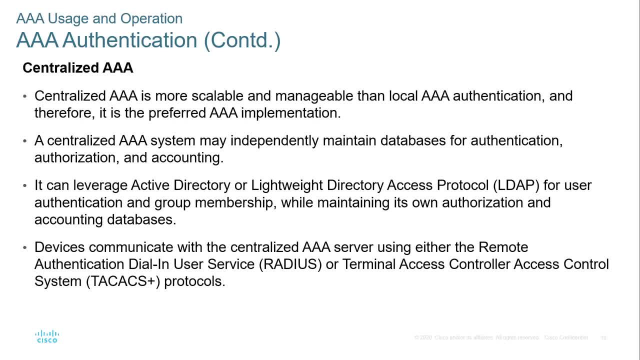 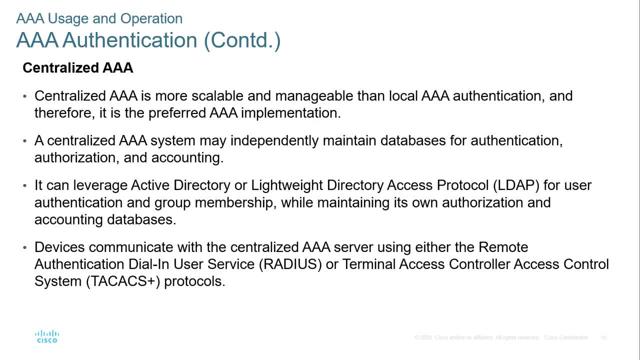 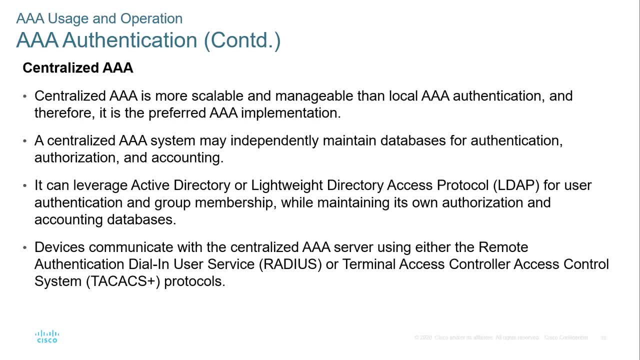 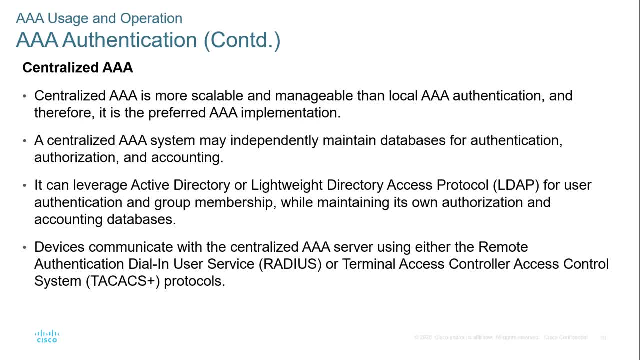 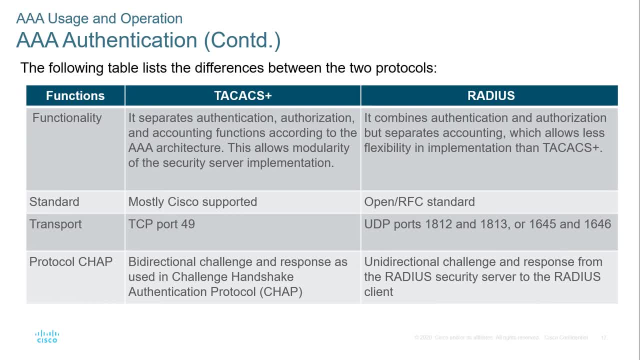 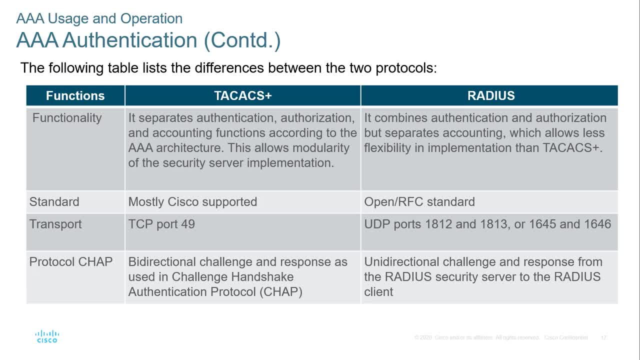 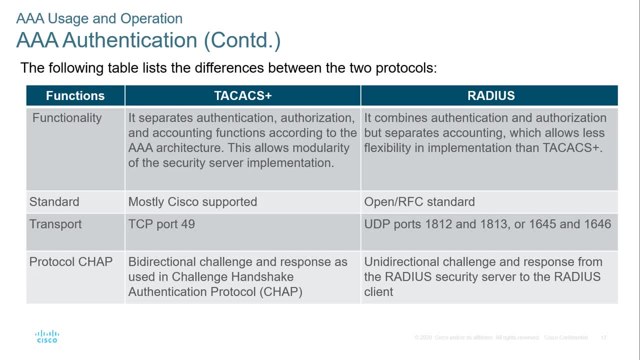 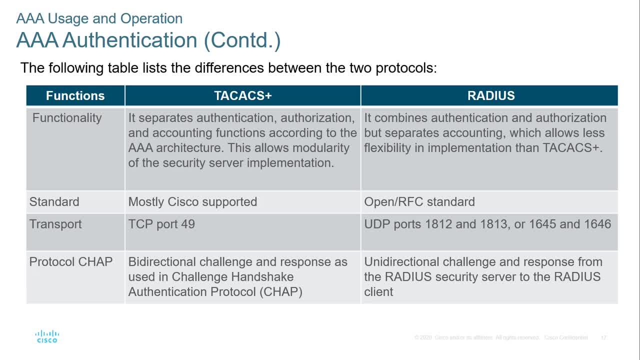 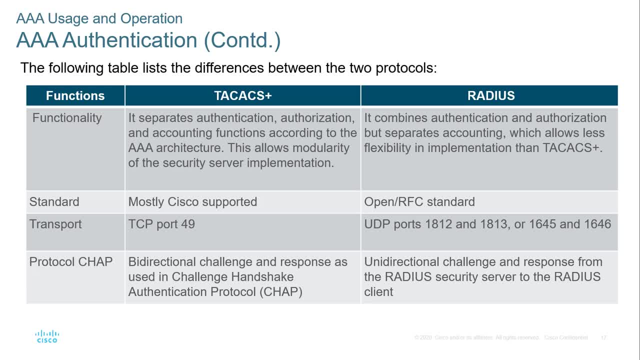 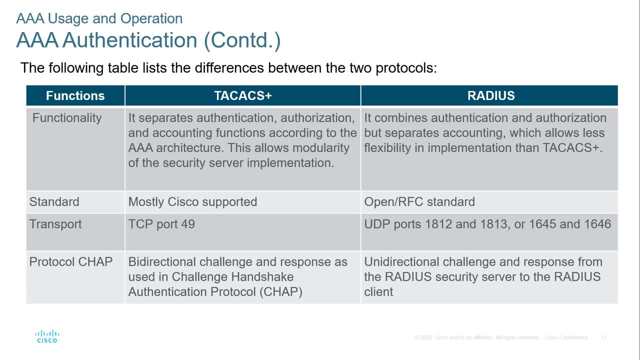 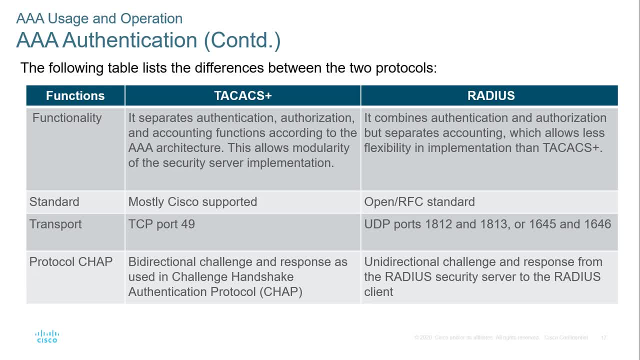 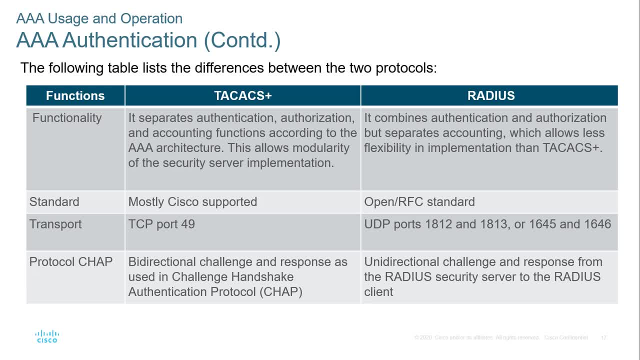 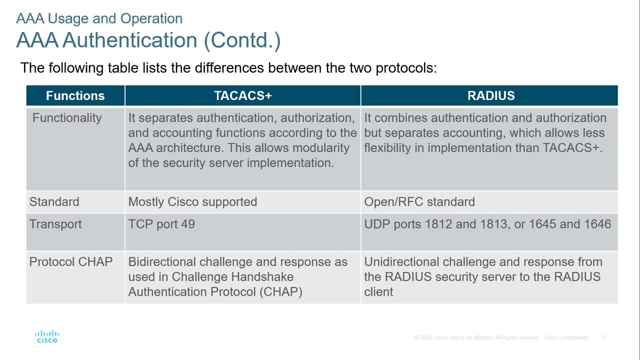 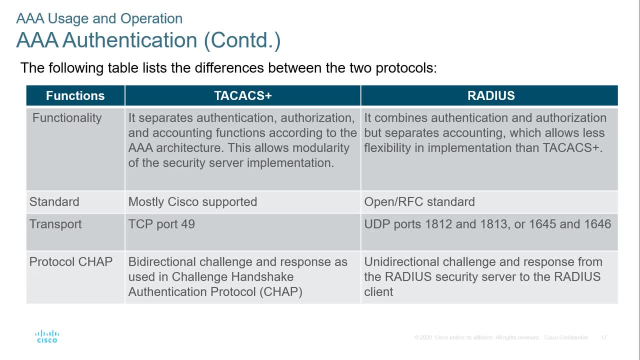 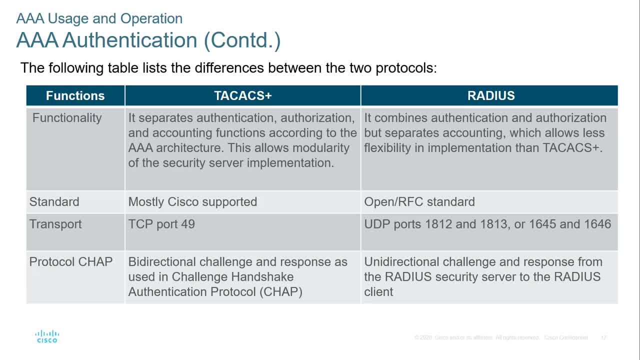 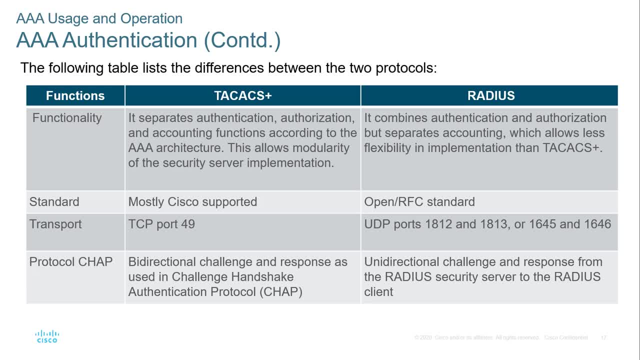 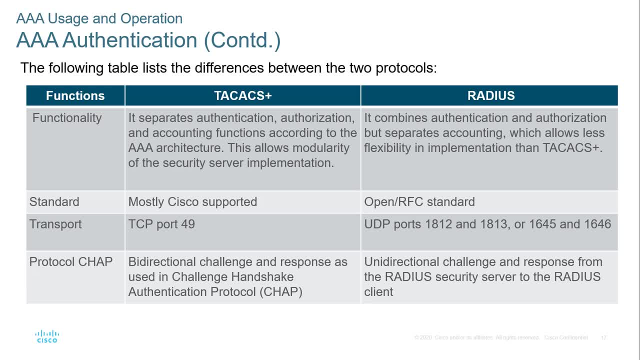 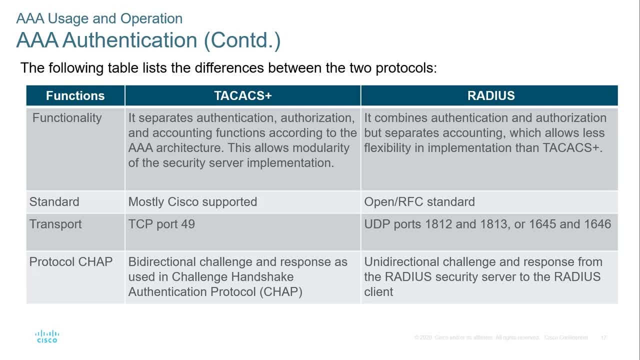 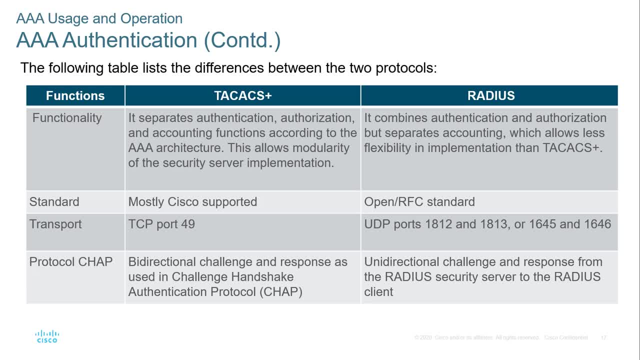 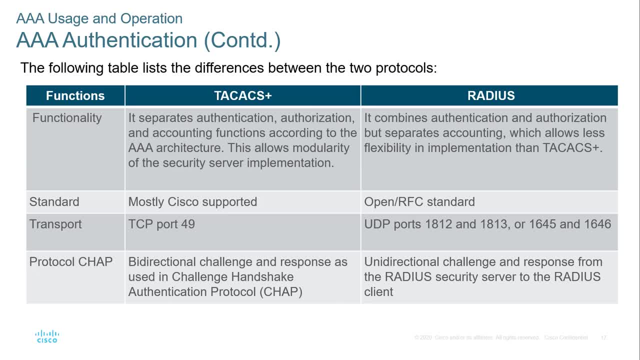 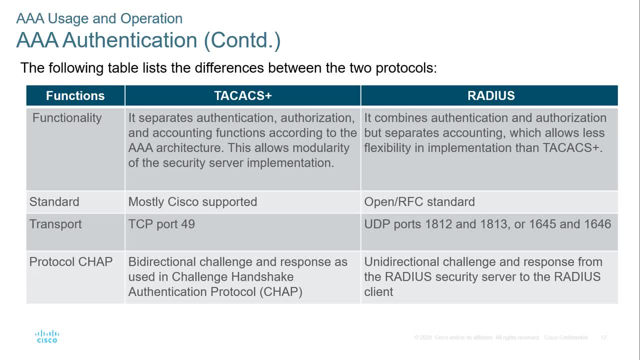 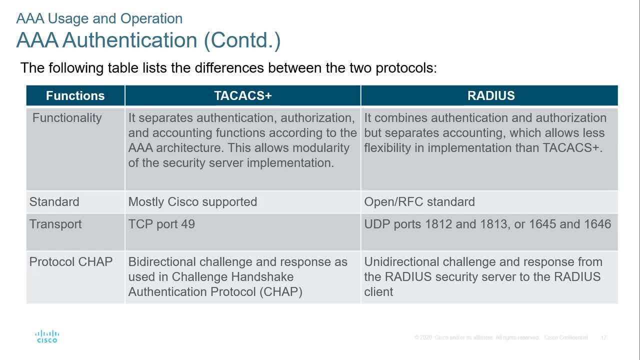 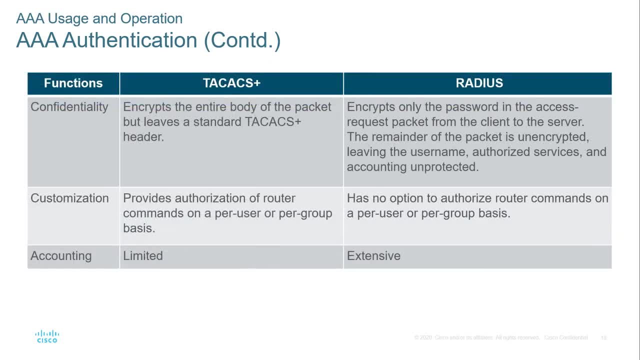 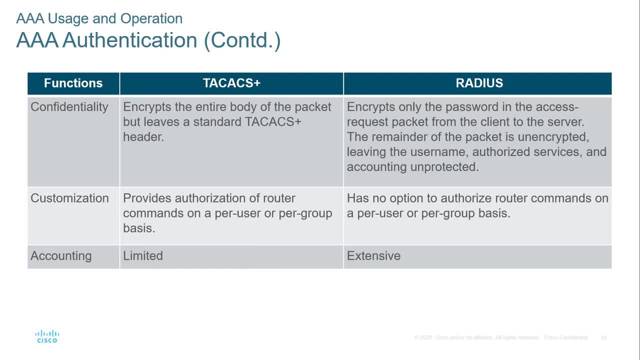 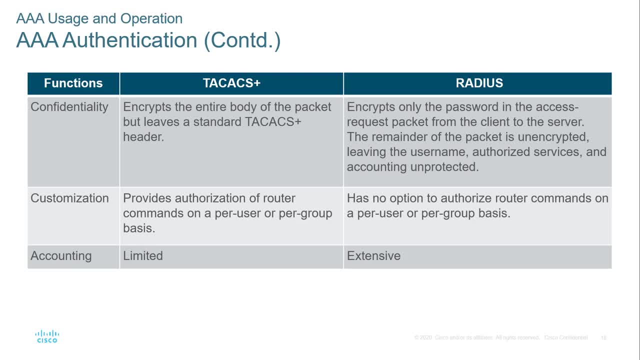 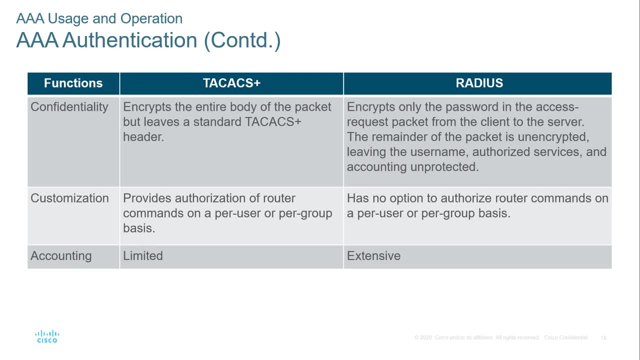 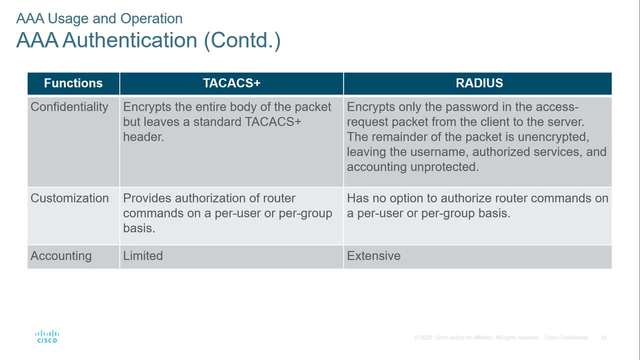 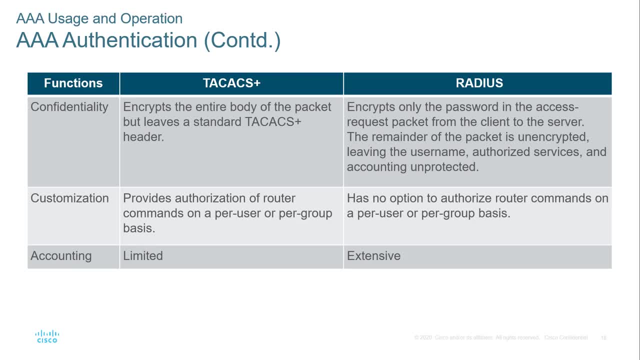 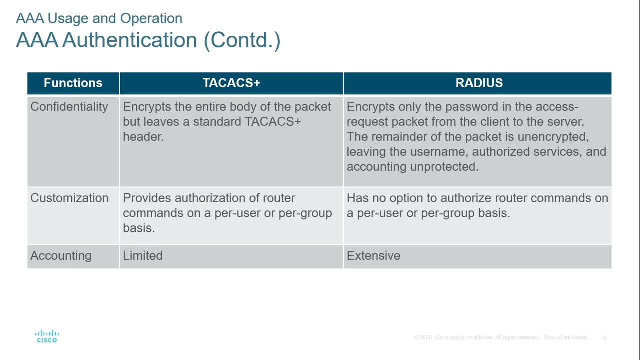 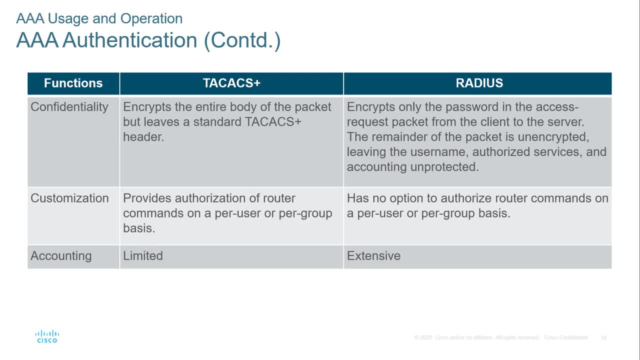 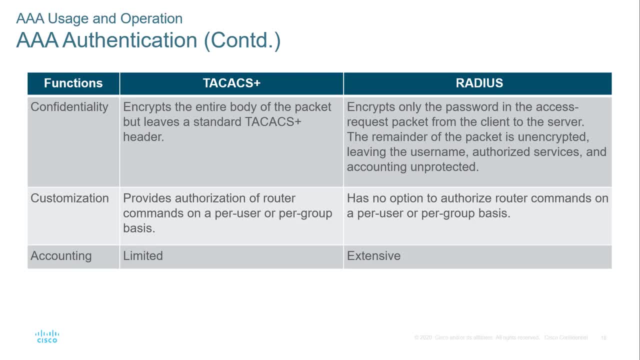 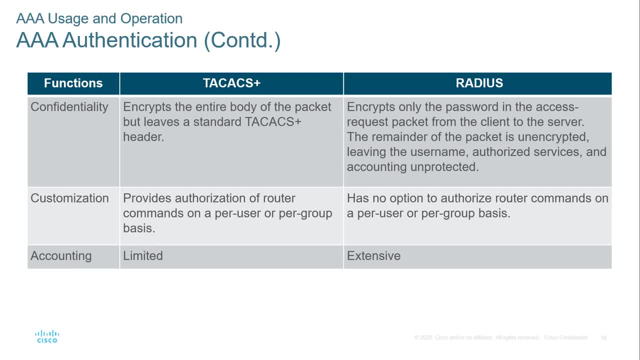 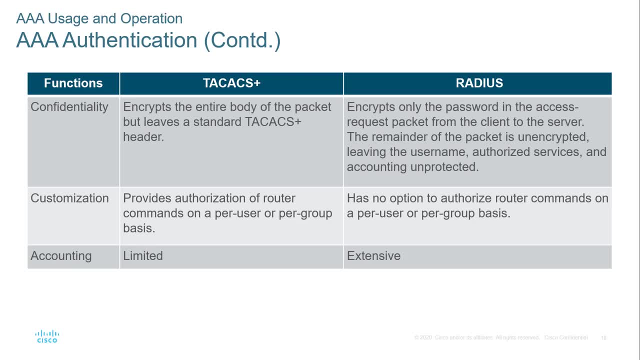 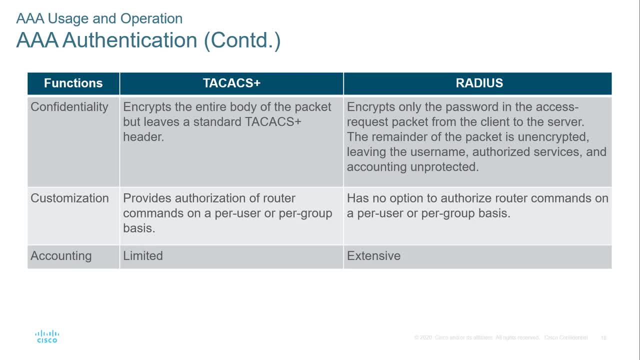 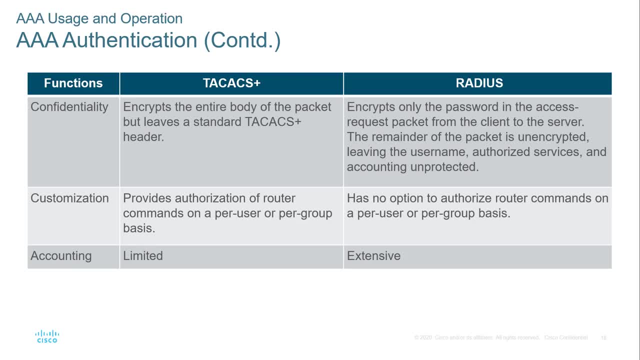 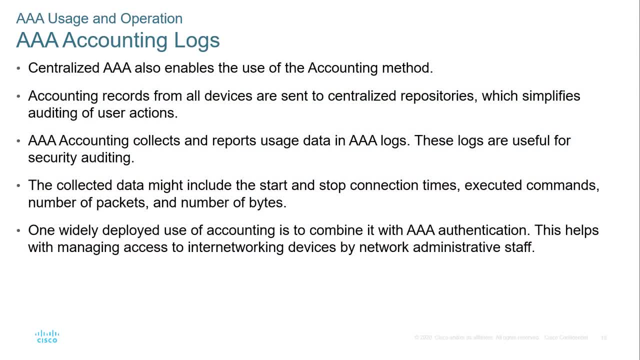 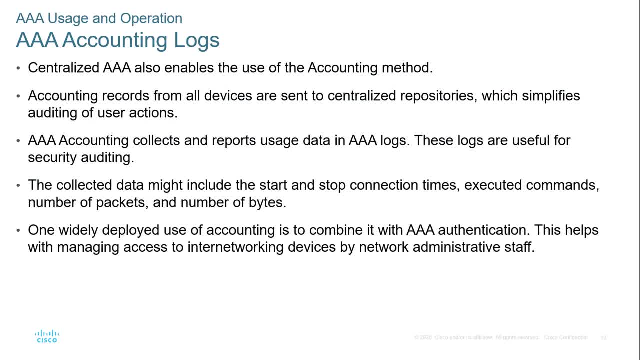 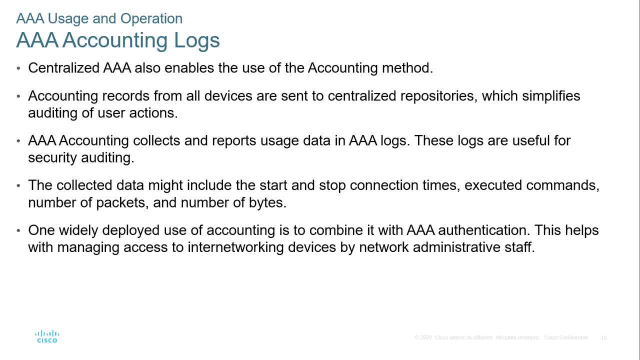 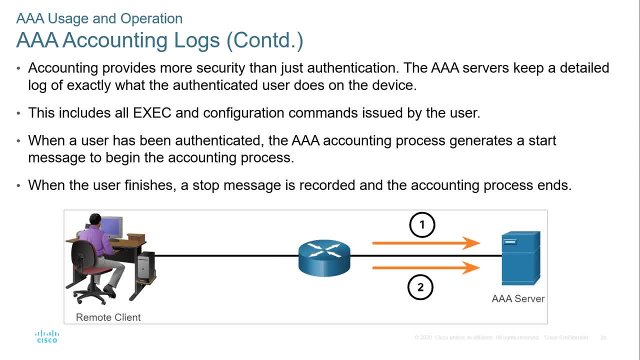 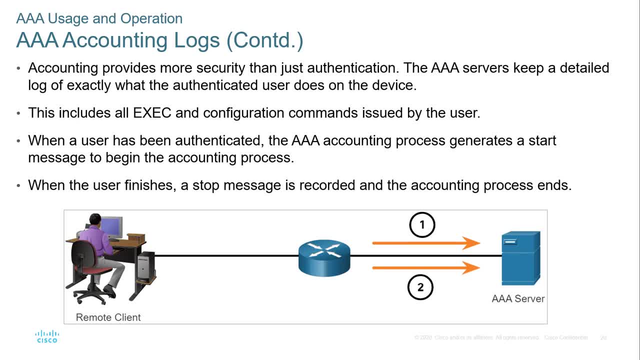 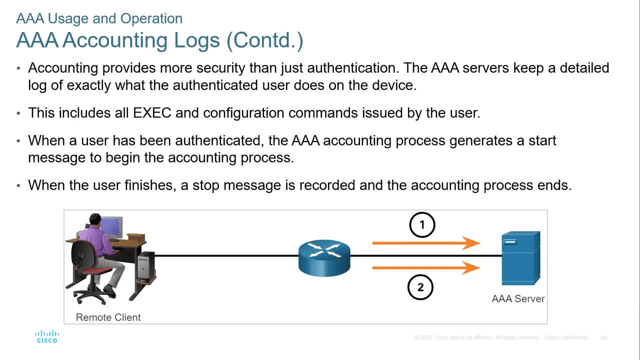 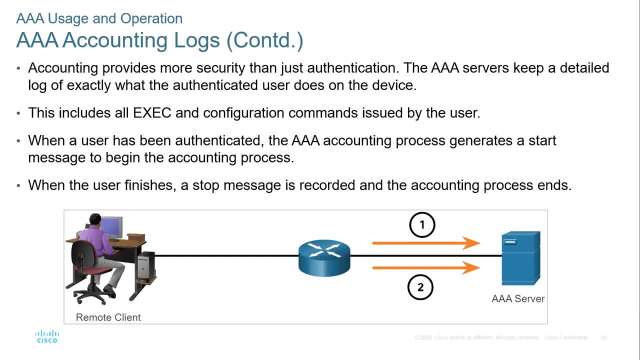 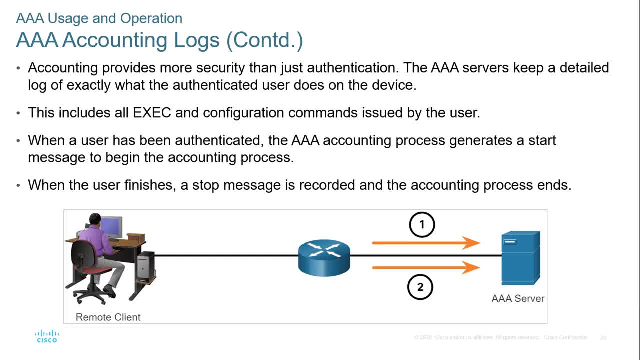 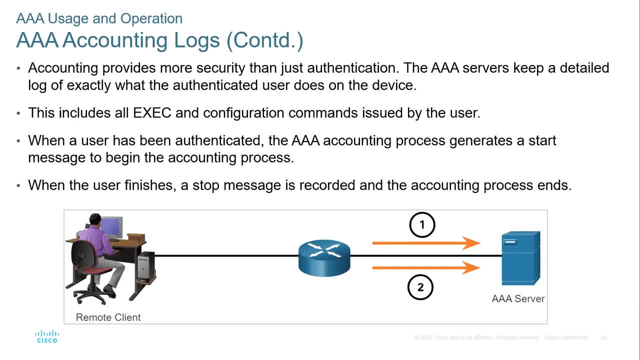 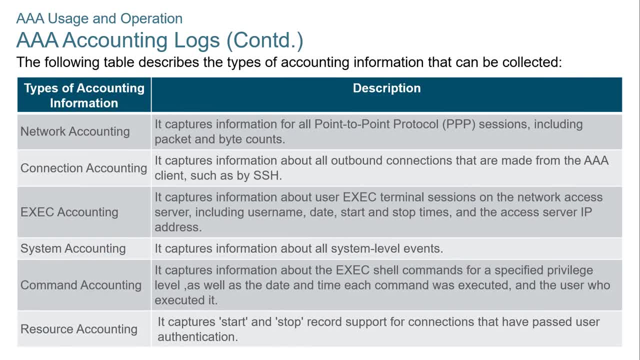 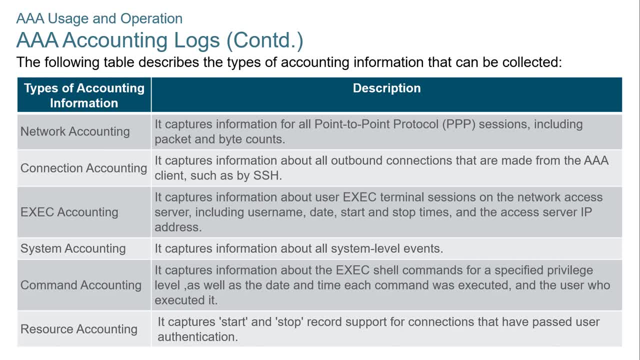 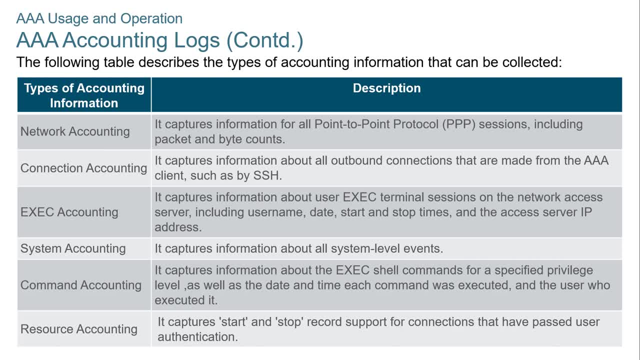 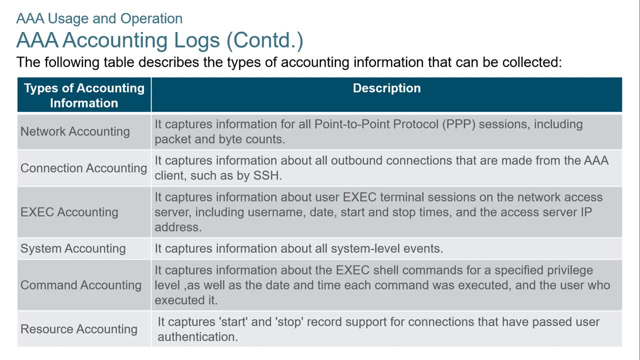 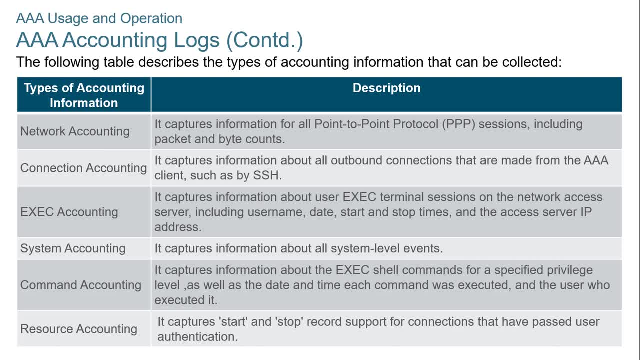 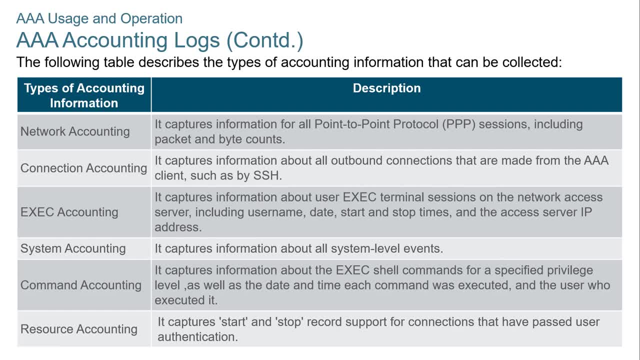 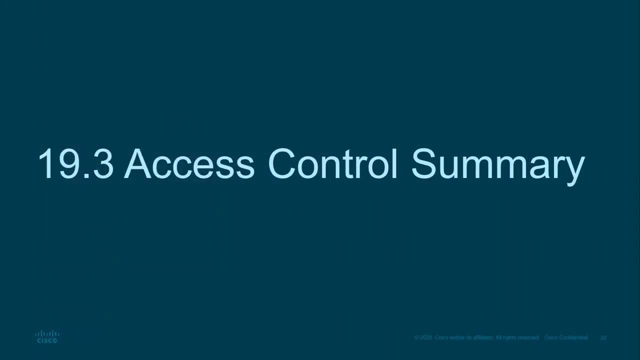 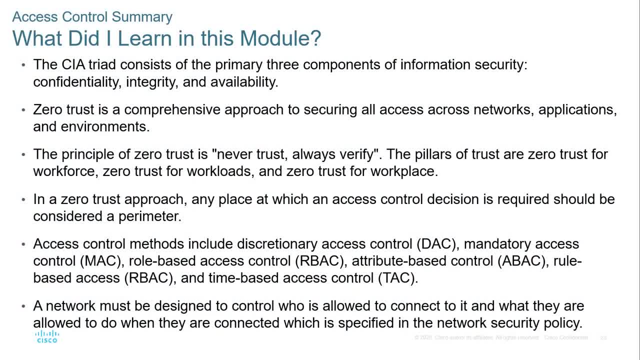